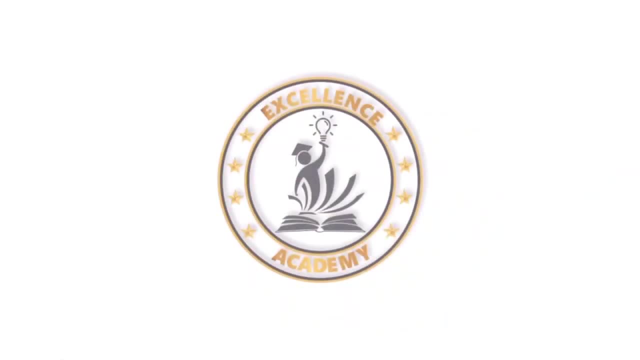 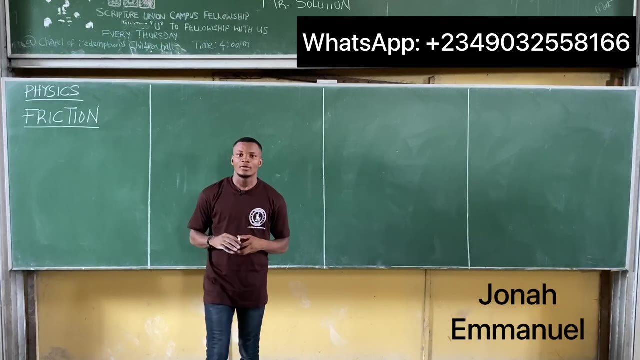 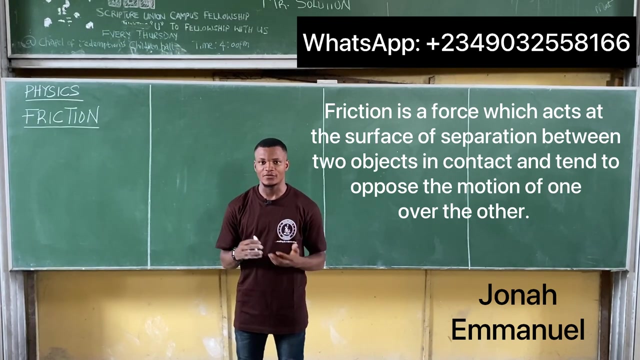 Welcome to today's class, For today we're treating friction By definition. friction is simply a force that acts at the surface of separation between two bodies and tends to oppose the motion of one body over the other. That's your definition for friction. 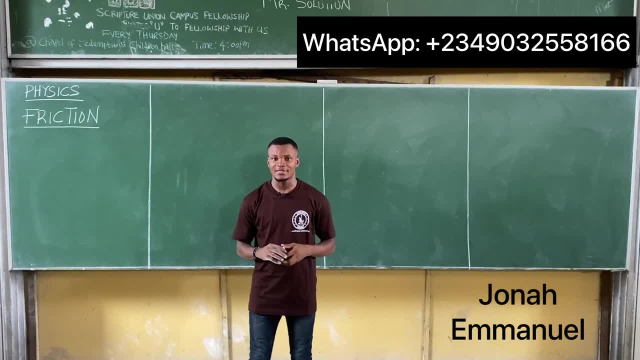 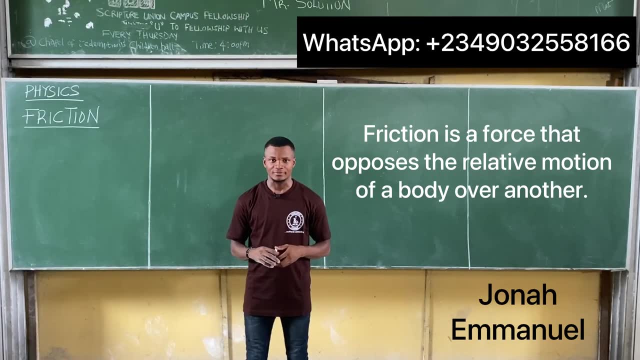 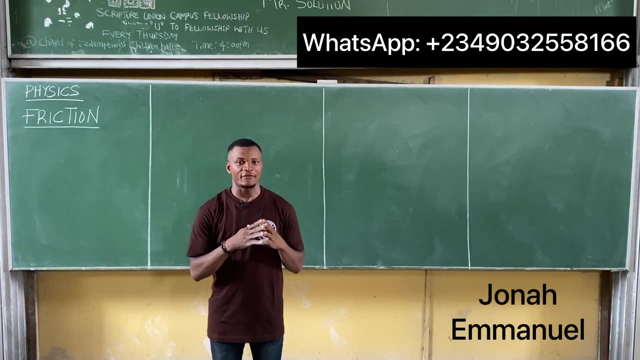 Alternatively, we can define friction as a force that opposes the relative motion of a body over the other. Now, from the definition there, there are some things to pick up from there. Number one is that friction is a force that opposes motion, And number two, it opposes 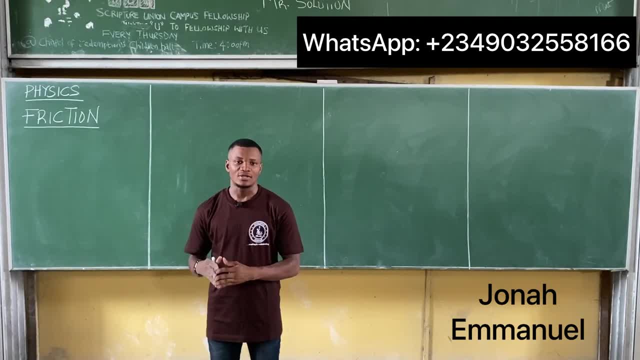 the motion of one body in contact with another body. That means for friction to occur. the motion of one body in contact with another body is a force that acts at the surface of separation between two bodies, and the body must be moving relative to another body. So 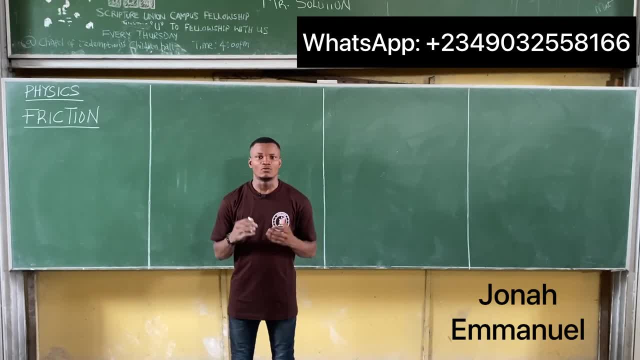 that's your definition for friction. Next up, let's look at where exactly does friction act Now? we said friction is a force And, from what we know, from an idea of vectors and scalar, we said force is a vector quantity And force being a vector quantity means it. 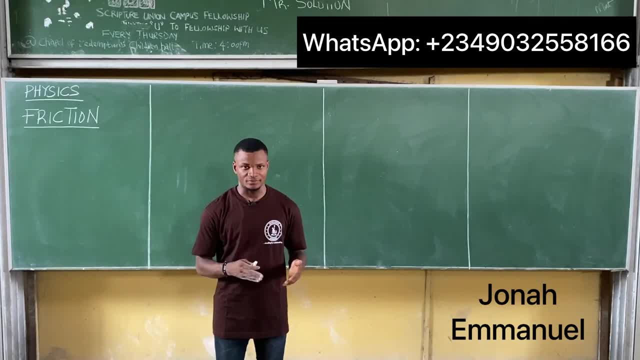 must have magnitude and then direction. But the question is: how do we know that? Well, the question is this: What is the direction of frictional force? Now, we said frictional force tends to oppose the motion of a body And hence, if it opposes the motion of a body, 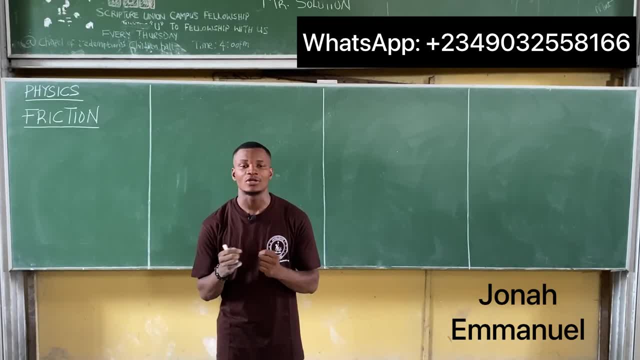 or for a force, perhaps friction, to oppose the motion of a body, it must be acting in the opposite direction of that body. Let's say, for instance: I have a surface like this. Let's use two scenarios. Let's say: I have a surface like this. Let's use two scenarios. 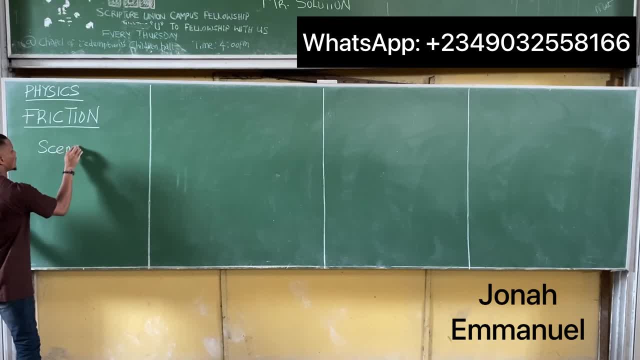 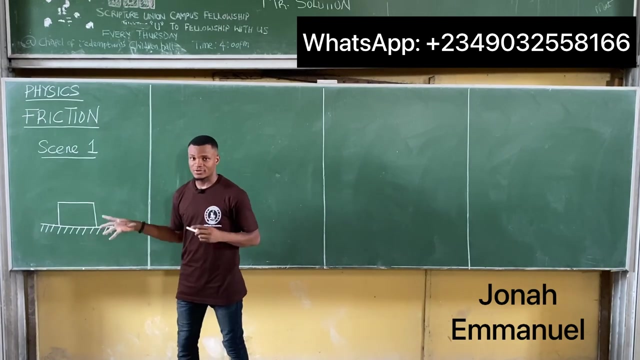 Let's say sin A or sin 1.. For sin 1, let's have a body on a surface. Let's use a rough surface, because if it's a smooth surface, friction will not really occur in smooth surfaces. So we'll do this, showing that it's a rough surface. Let's have a left. All right Now. 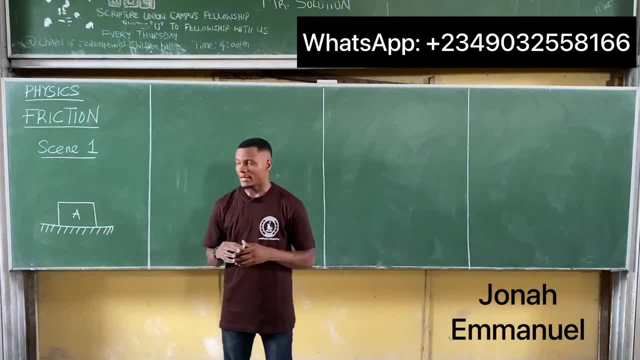 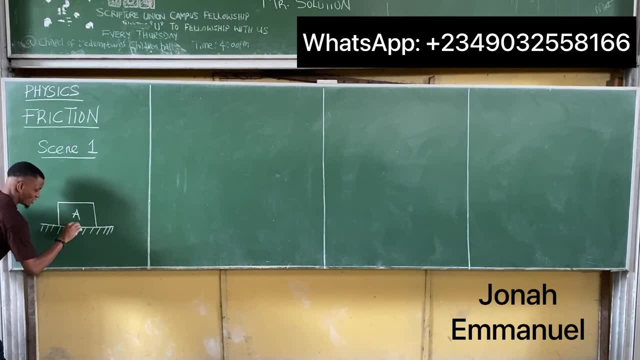 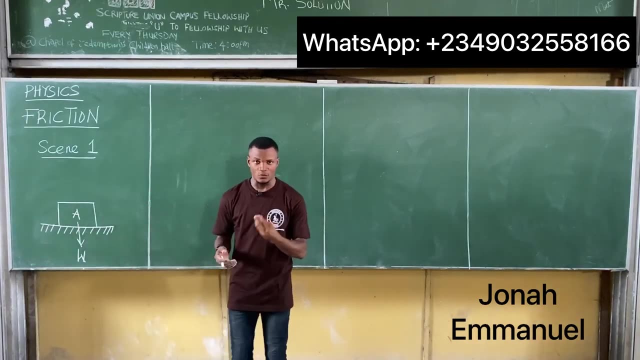 what is body? For a body resting on a rough surface, two forces acts on this body. The first one there is the weight of the body. Of course, the weight of the body acts downward, So you have weight acting downward. For a body resting on a rough surface, the weight acts downward. 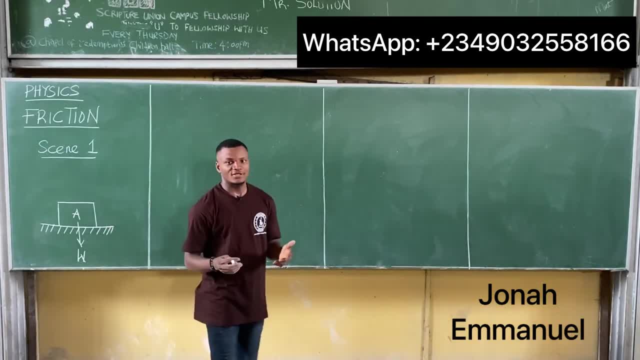 Next up from Newton's thought of motion. it says: to every action there's an opposite and equal reaction. So the force I have to balance this. Let's say sin A or sin 1, let's have this That has to balance the weight of the body. It's called the normal reaction. 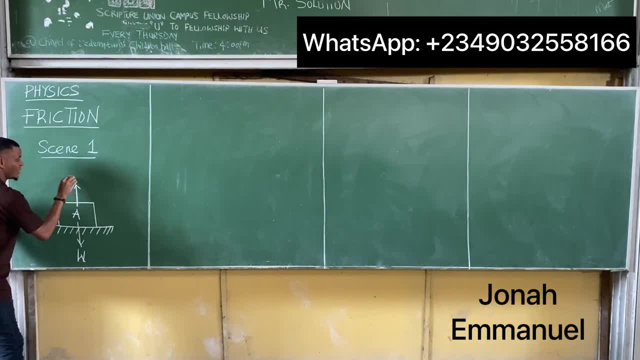 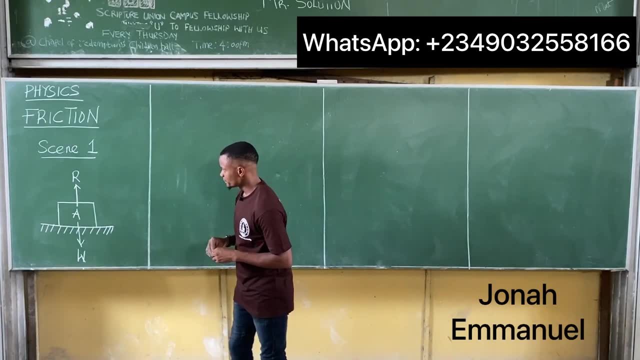 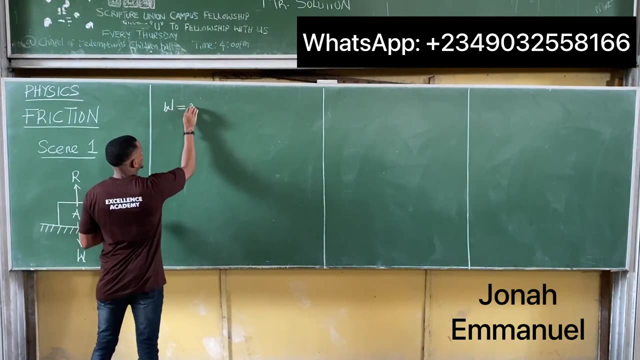 So the force here that will balance this is called the normal reaction. We'll call this A, So technically we can use N. All right, Normal reaction. that's A or N. Okay Now, so we have this. So we just said that W. we just said that W is called the weight. 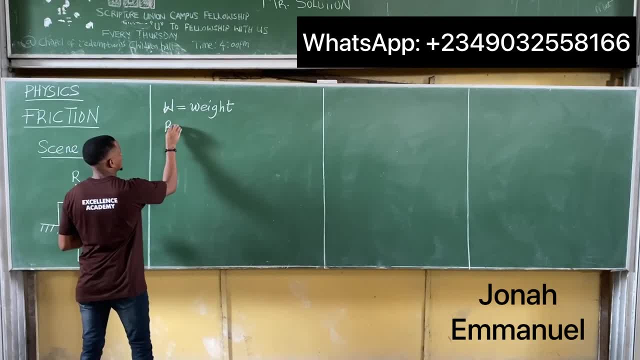 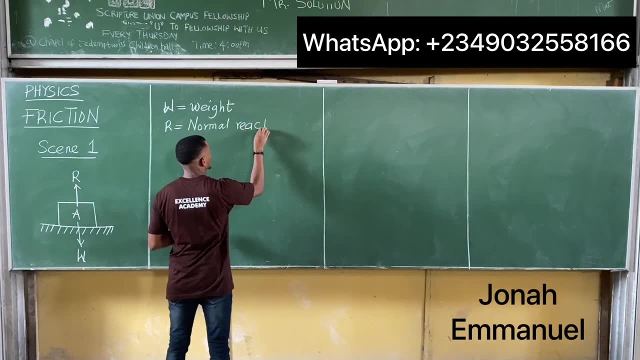 of the body. Why A? Why A? Why A? Because this A was shown by Newton. The weight, we said, is the normal reaction. Of course weight is measured in Newton. Normal reaction is also in Newton. Both of them are in Newton. In some cases, in certain texts, they call normal reactions. 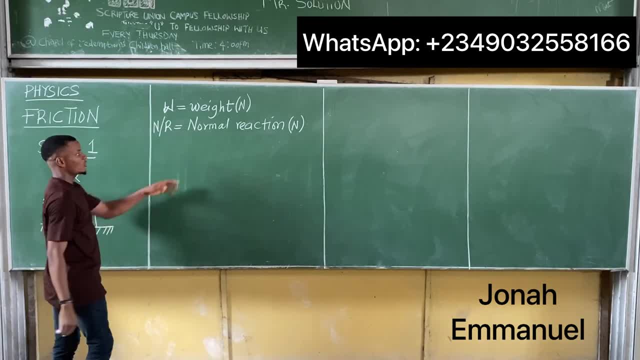 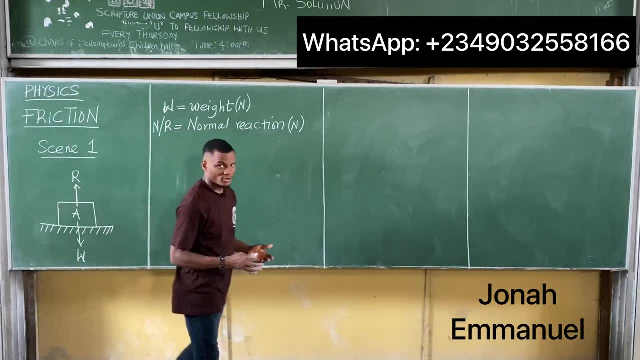 N. So now you want to call normal reaction as N or I, It's the same thing. Okay, All right. So for this body now moving. so here's the thing in this body. let's say it moves towards the left. if the body moves, this: 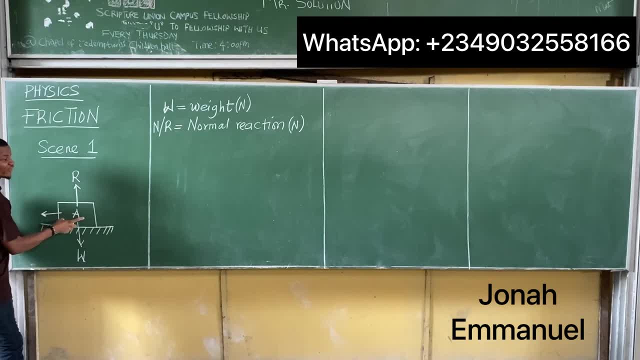 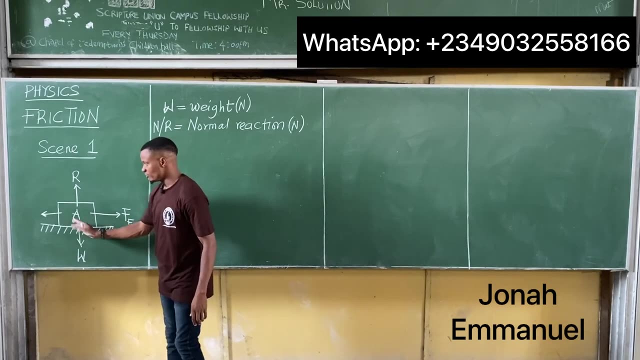 way here. of course, to oppose the motion of this body, i will have to move in the opposite direction. so hence, if this body is moving to the left, the functional force will move to the right. so i have this all right. this is a c8 says: if the body is moving towards the right, left, to oppose the 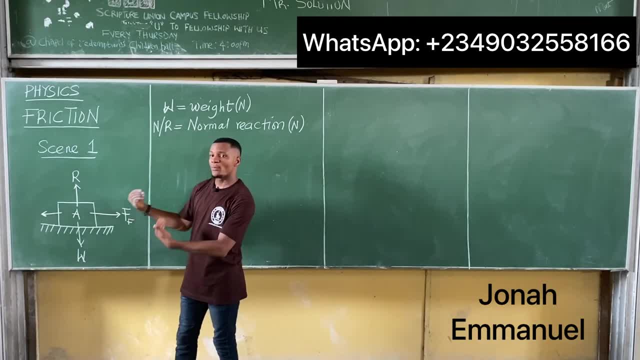 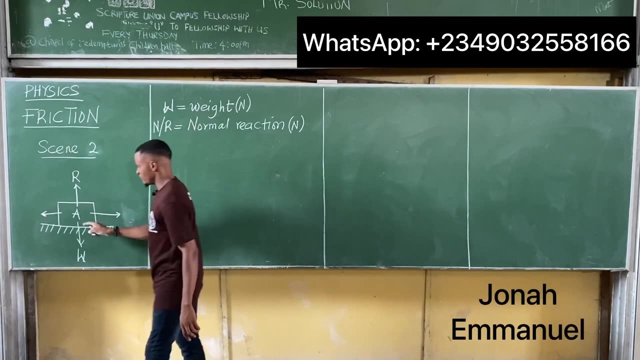 motion of this body, the fictional force has to act in the opposite direction, according to newton's third law, and hence fictional course goes to the right. that's the one, same two, same two. what if we revise the case? what if the body moves to the right? obviously for friction, of course, to. 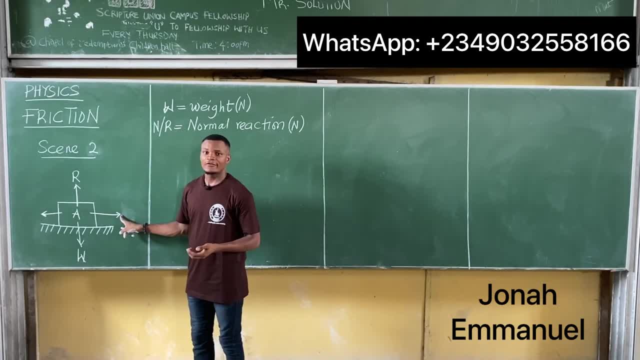 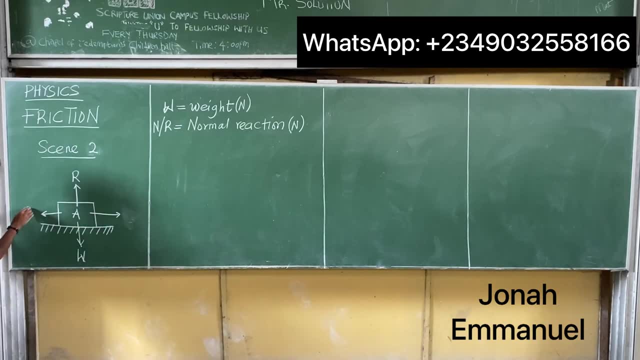 oppose the motion, it has to move in the opposite direction. so hence, if the body is moving towards the right, the fictional course will move towards the left. so i have this. so these are like two scenarios where fictional force works. so the idea is very simple: fictional force will always act in. 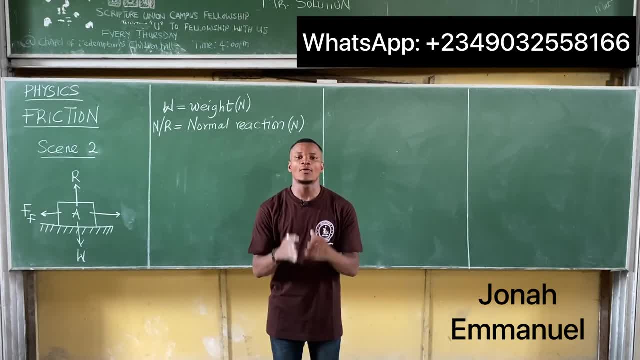 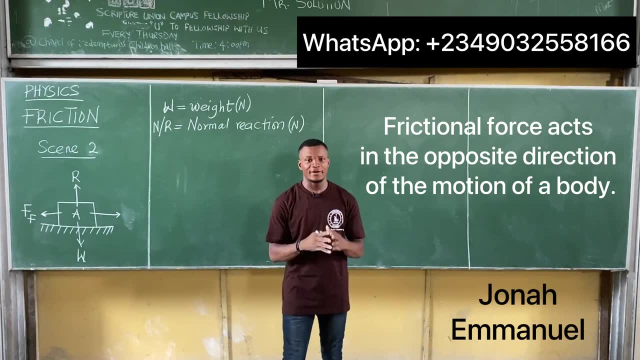 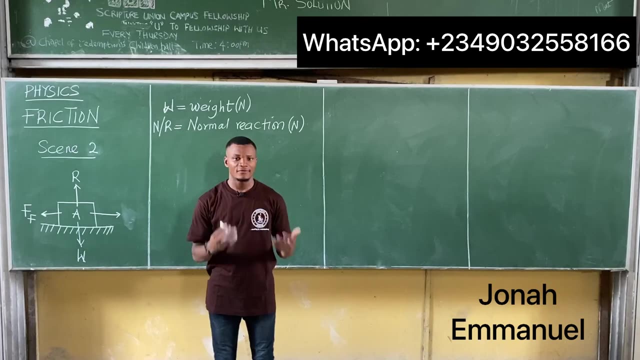 the opposing direction of the motion of a body, that is, the direction for fictional force. so now let's go to the next one. so this is a c8. so if the body is moving towards the right. having considered this, let's look at the types of fictional forces that we have. 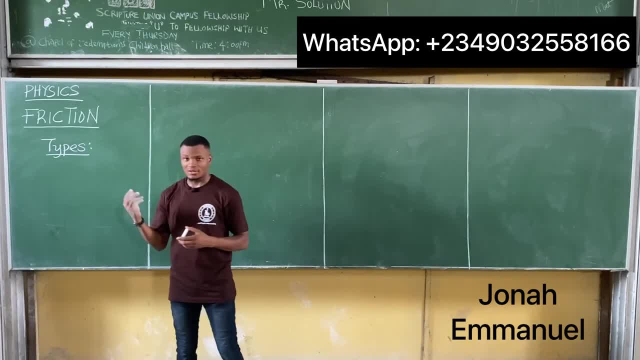 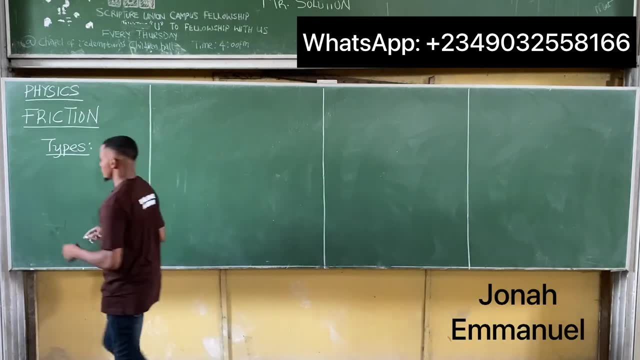 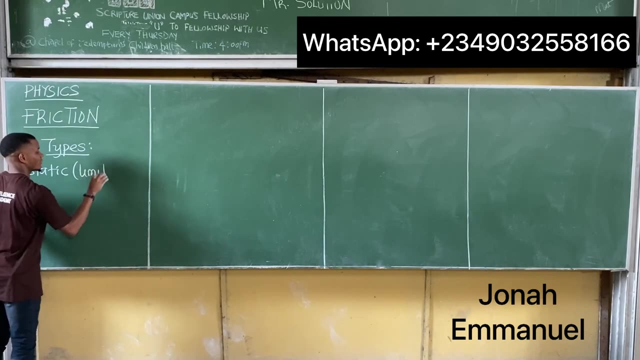 so next up, let's look at the types of fictional forces. there are two types of fictional forces. the first one is called the static, also known as the limiting original force. the second one is called. the second one is called the kinematic, also known as the dynamic fictional form. 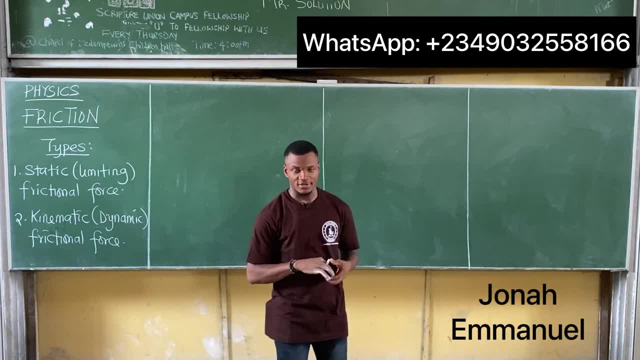 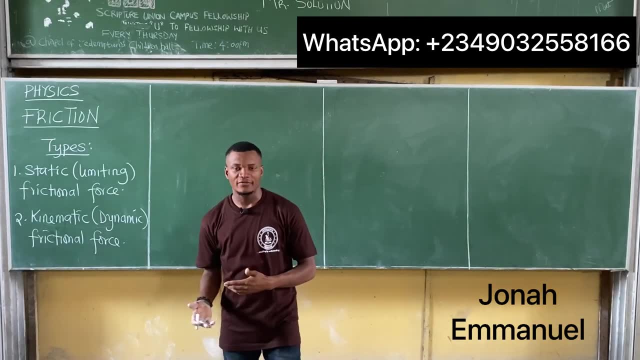 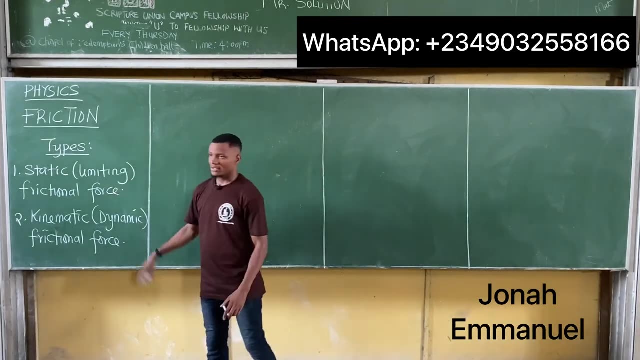 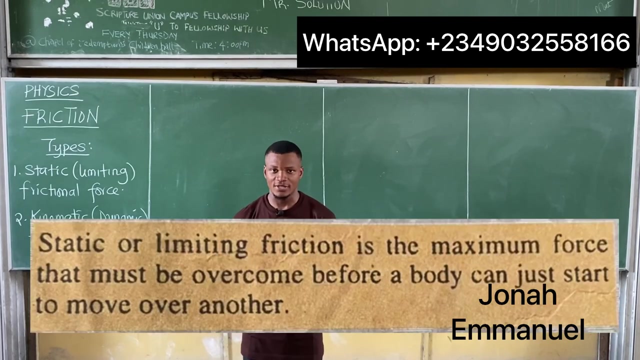 all right, let's consider these two fictional forces and what they mean. all right, so, uh, we said that the final force, the static, also called using fictional force, and also the kinematic, also known as dynamic fictional force. what is static or limiting fictional force? static or limiting fictional force is the maximum force that must be overcome before a body can just start. 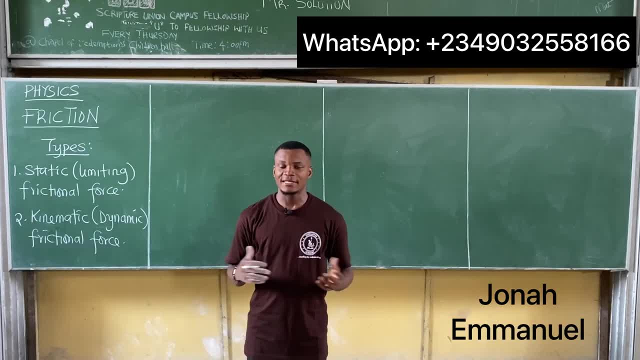 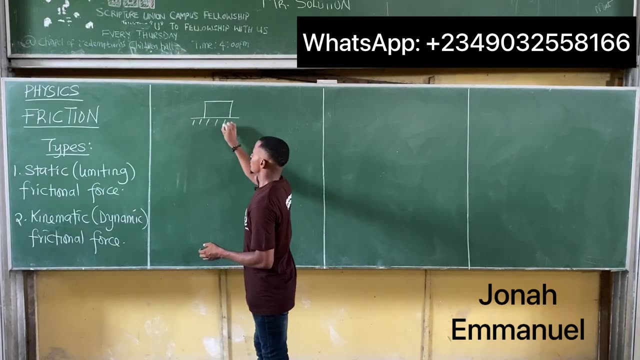 to move over another body. that's enough. that is static or limiting fictional force. for example, if i, If I have a body as I drew earlier, if I have a body on a rough surface as this, The maximum force that must be overcome before this body can just start to move over this surface is known as the static frictional force. 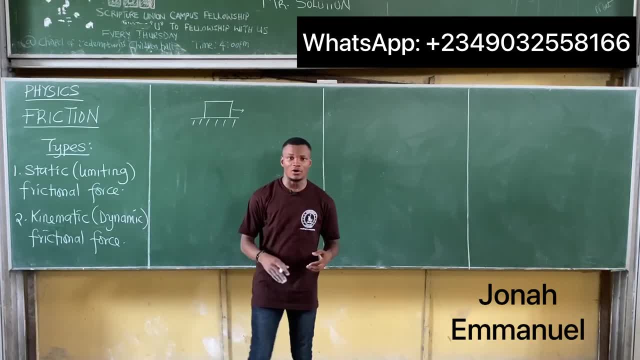 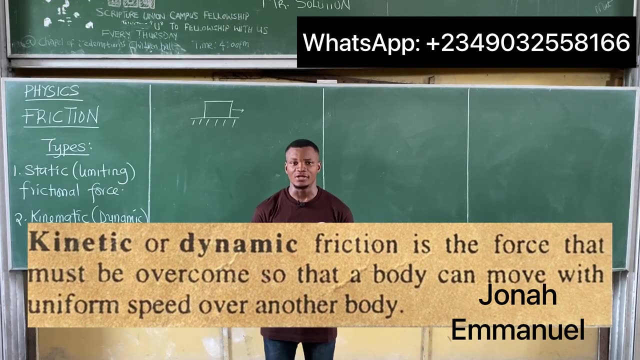 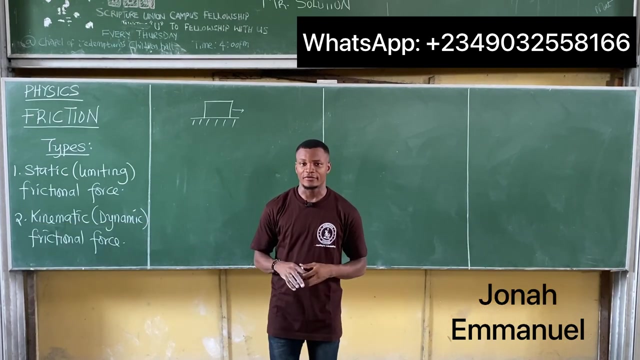 This is case one. Next up, let's look at kinematic or dynamic frictional force. By definition, kinematic or dynamic frictional force is simply the force that must be overcome before a body moves with a uniform speed over another body. That is kinematic or dynamic frictional force. 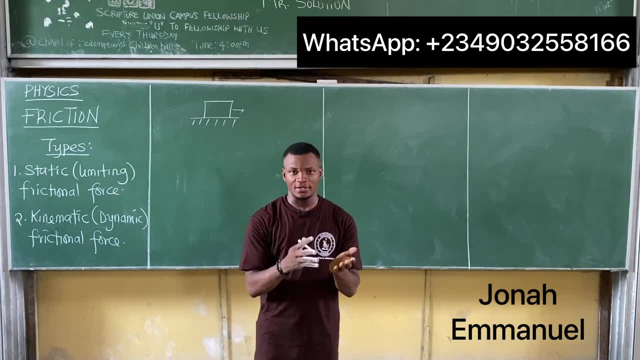 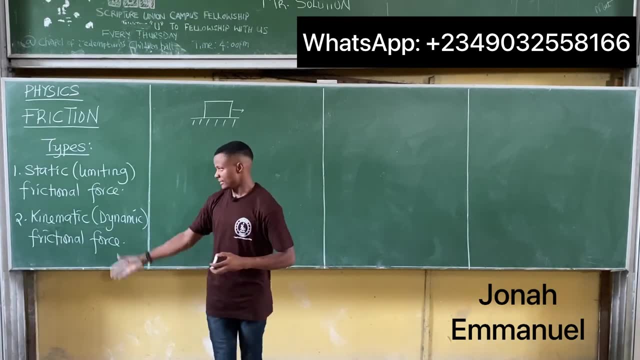 So the force responsible for placing a body in uniform speed over another body is what we call kinematic or dynamic frictional force. So the force responsible for placing a body in uniform speed over another body is what we call kinematic or dynamic frictional force. 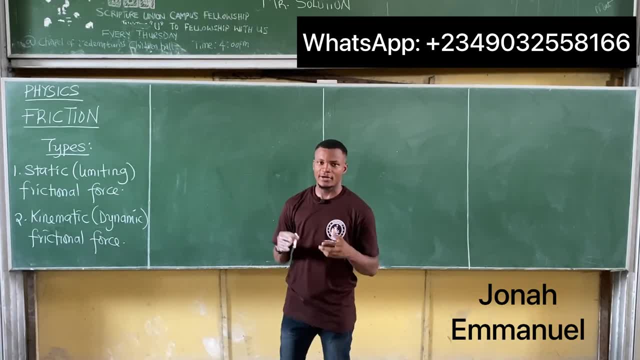 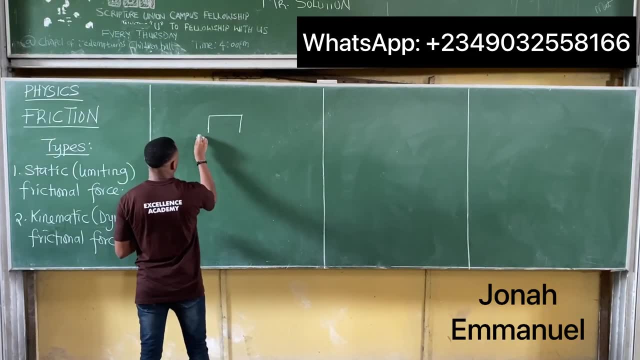 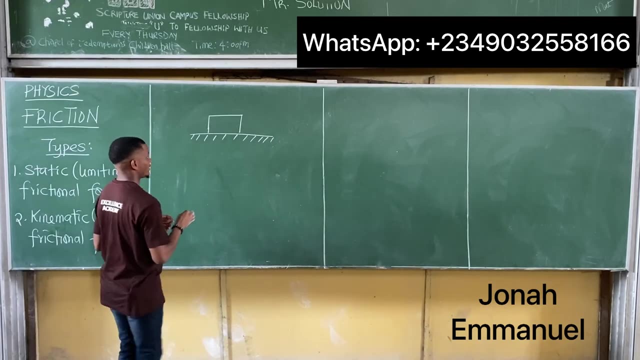 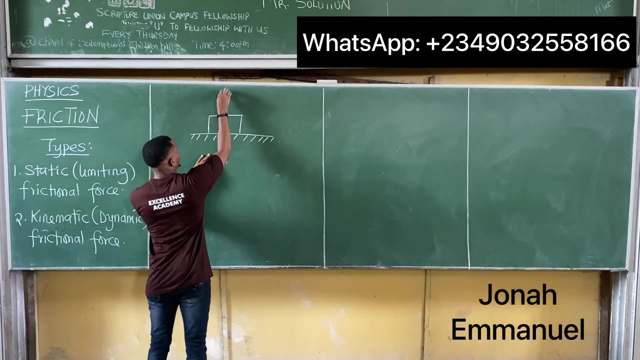 Alright. so, having considered this, let's look at a concept in frictional force. Now, we said, when a body is placed on a rough surface like this, we said, the forces that act here include, number one, the weight coming downward. Number two, the normal reaction going upwards. 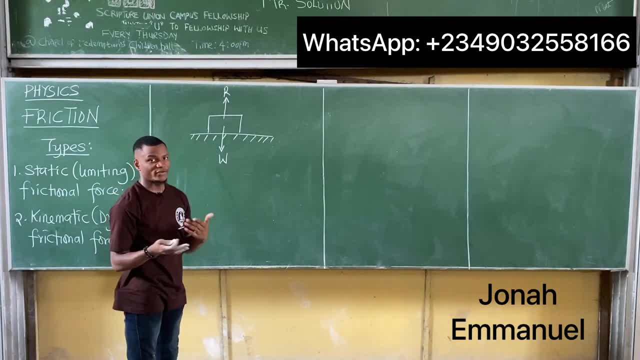 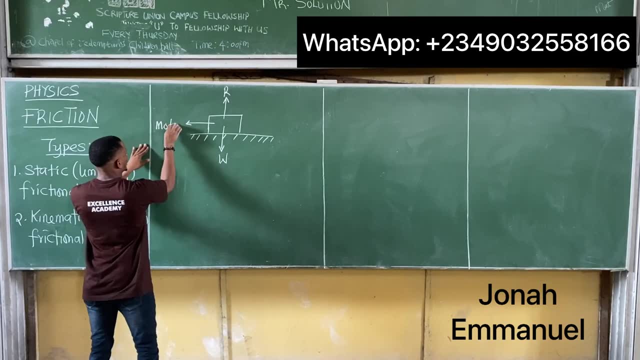 Number three: depending on the direction of the motion of the body. if the body is moving this way, if this is the direction of the motion, then we said frictional force FF. So if this is the motion of the body, then the frictional force acts here. 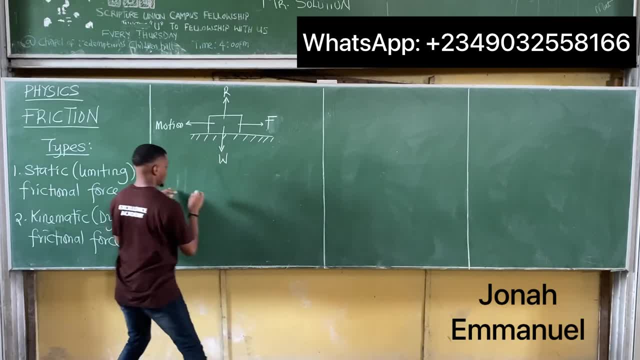 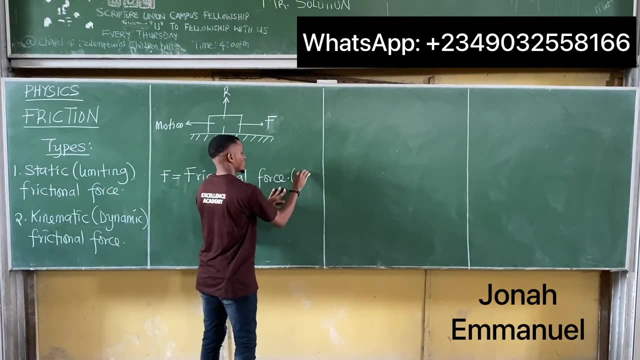 Let's call this F Please. F here is frictional force. Let's indicate that F is equal to frictional force. Frictional force- We have this, of course, also in near-term. Of course, force in near-term. 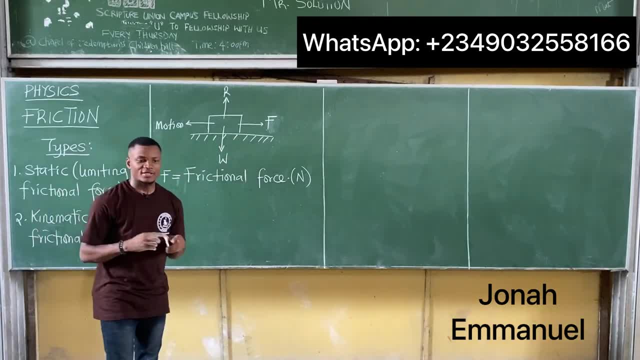 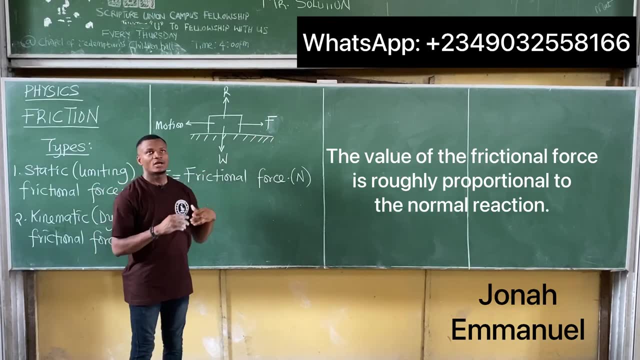 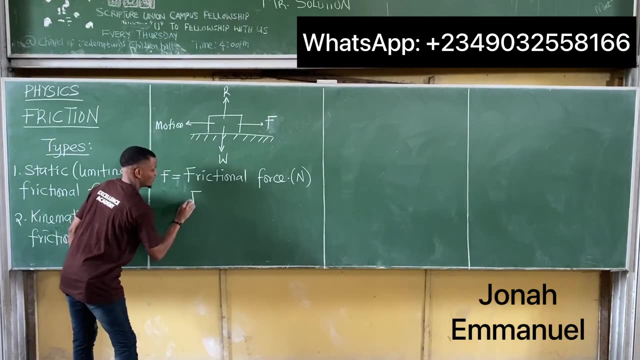 So we have frictional force in near-term. Now, having considered this, let's look at something. From experiments it has been seen that the value of frictional force is roughly proportional to the normal reaction. So frictional force you can say roughly it is proportional to the normal reaction. 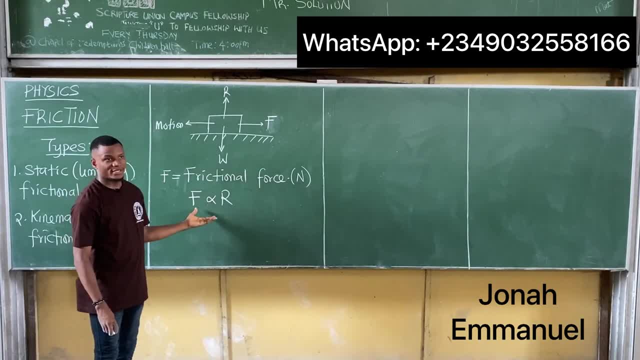 So we have this And from the idea of mathematics we said: whenever you have a proportionality sign, we take out that sign and introduce a constant. Of course, equal to and a constant. So that means the frictional force changes to equal to. 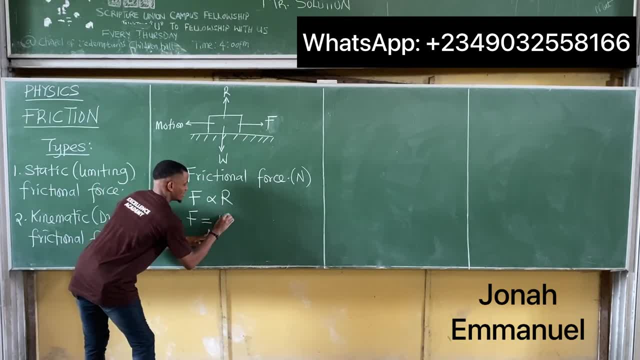 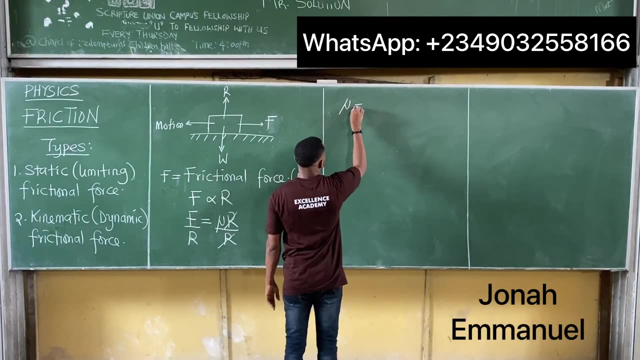 My constant in this case becomes mu, then F. If we have mu here, if I let mu subject to the formula, I will have to divide here by F, Divide here by F And these particles, So this mu is equal to F over I. 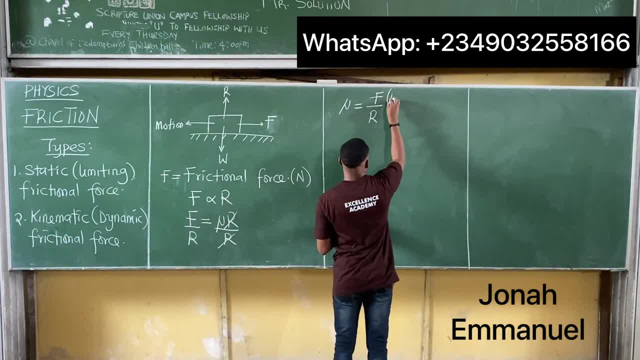 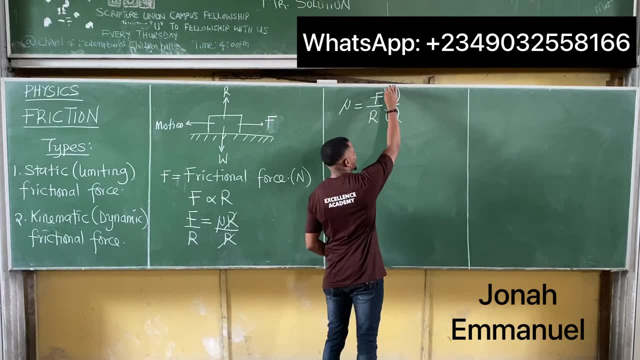 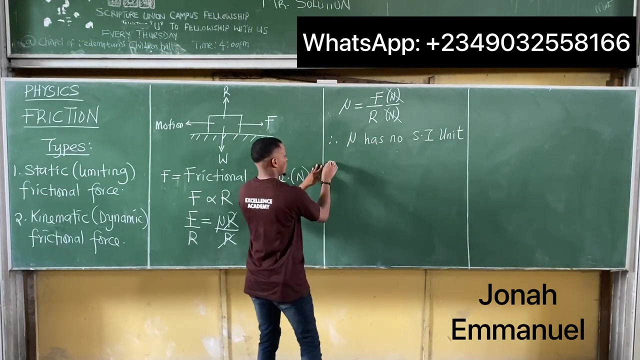 Let's include units. We said force is measured in Newton, Normal reaction also in Newton. So this is a case of Newton counting out. So therefore this mu has no SI. So it happens. Anyway, this is called mu. 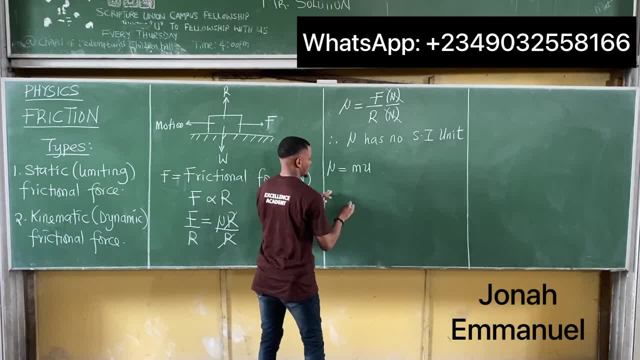 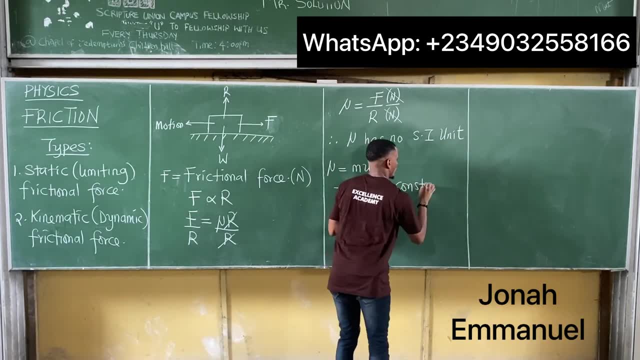 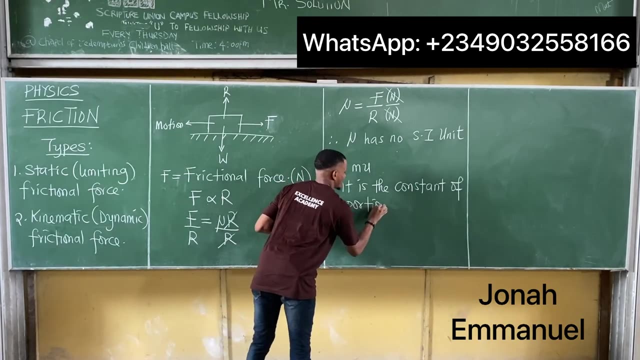 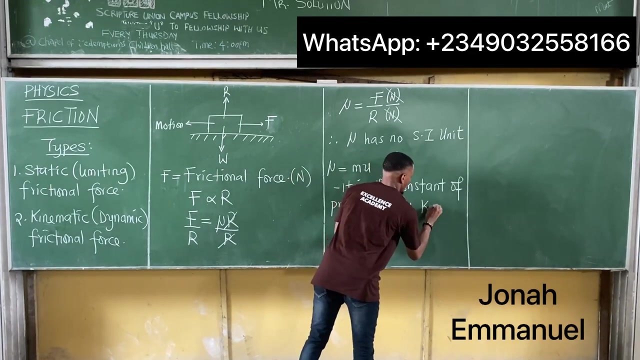 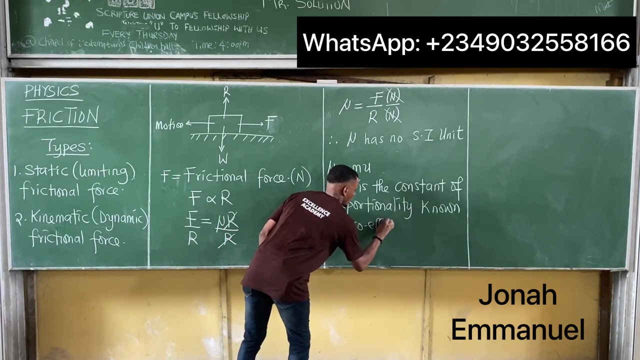 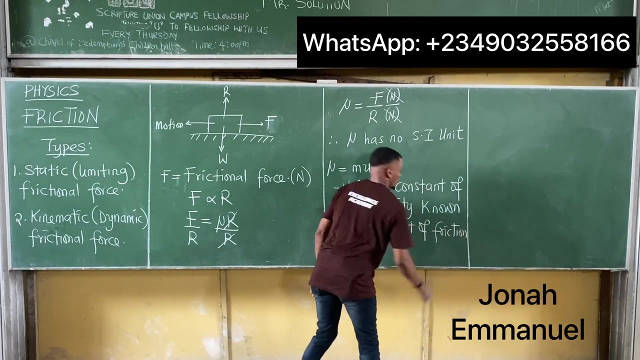 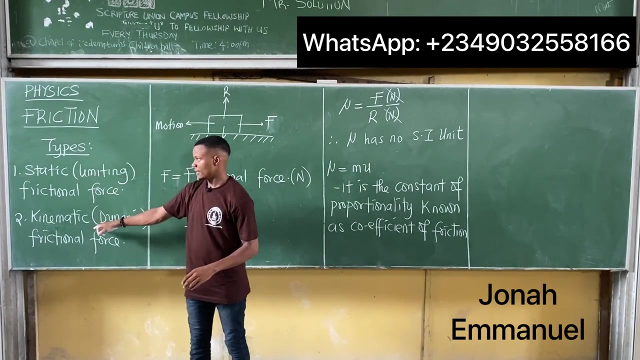 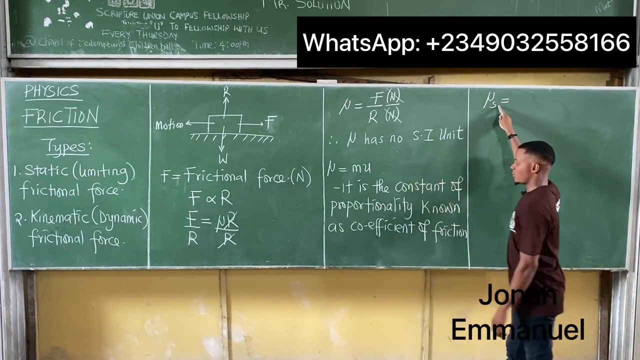 Pronounced mu. This is the constant of proportionality, Mu, Mu Known as coefficient of friction, Known as coefficient of friction. Now, mu exists for both static and kinematic. For static, you have mu S. This is called the coefficient of static friction. 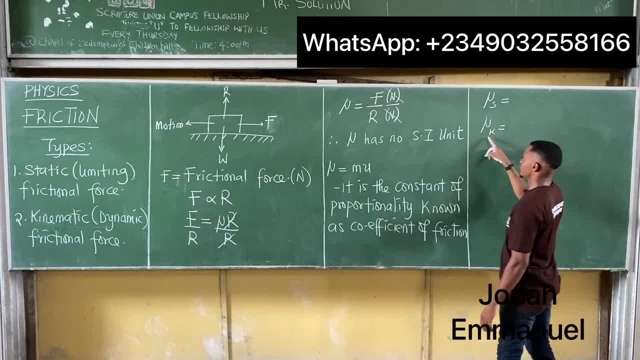 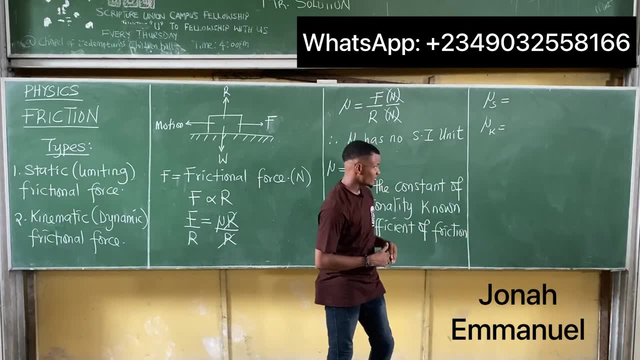 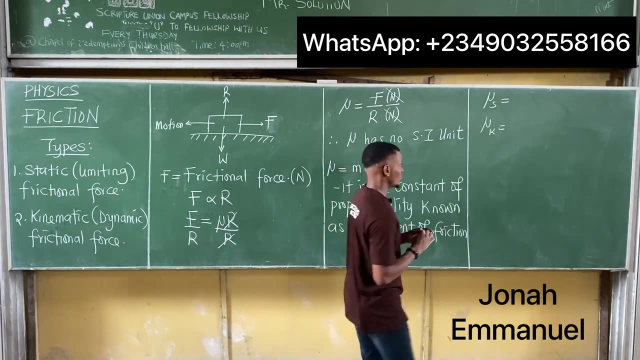 And we have mu K. This is called the coefficient of kinematic friction. That's it. So we have this concept, Alright, So we use this concept in solving some examples. But before that, it is important that you know that. 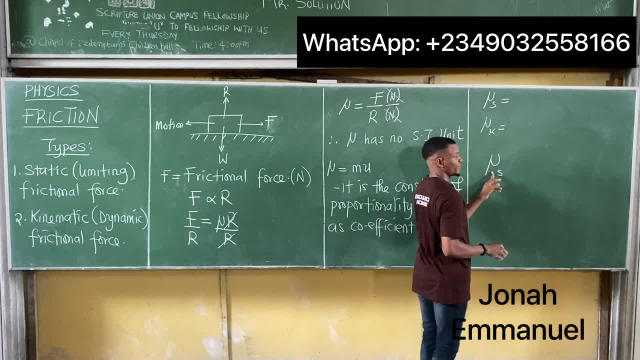 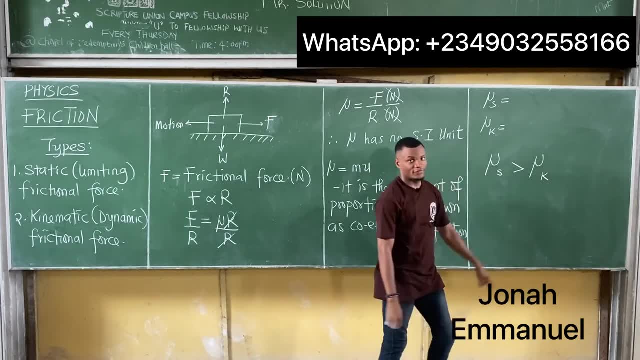 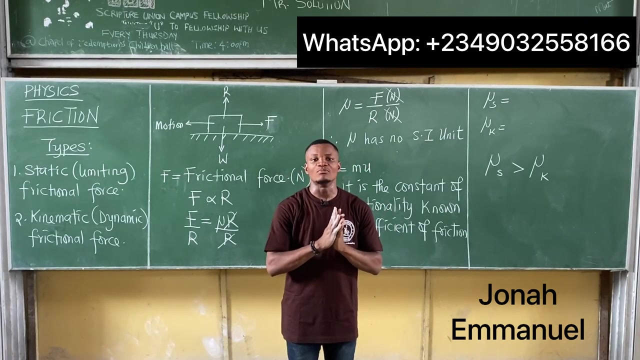 the value of the coefficient of static friction is greater than the value of the coefficient of kinematic friction. This is because more force is needed to make. We say for static friction that it is the maximum force that must be overcome before a body can move. 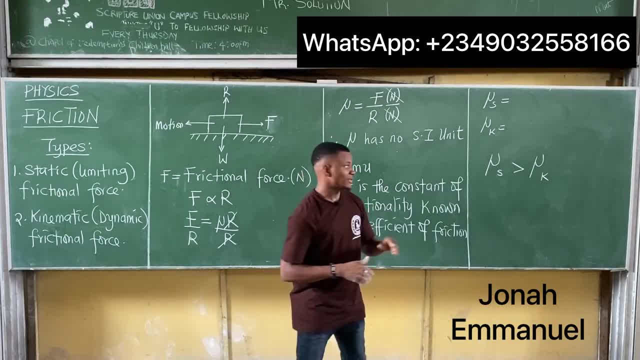 or can start moving over another body. And we said for kinematic friction that we said it is the force that must be overcome for a body to move with uniform speed over another body. Now it's quite obvious that more force is required for a body to start moving. 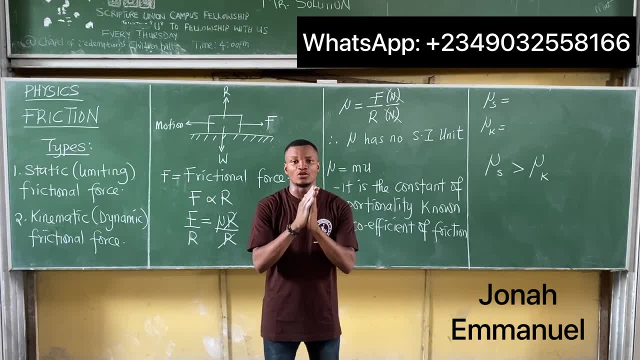 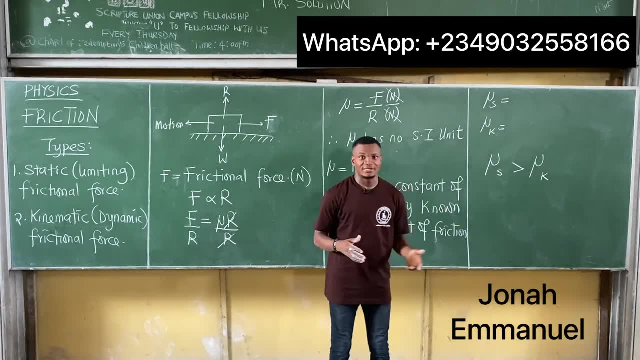 than is required to place a body in uniform speed. So I need more force right to push a body that is addressed to start moving than I need to make a moving body to move with uniform speed. So for this reason, since I need more force to move the body from rest, 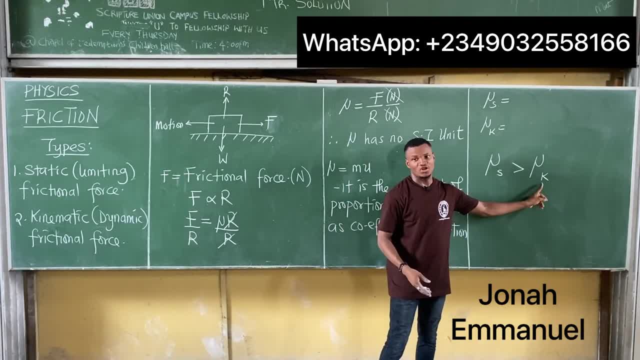 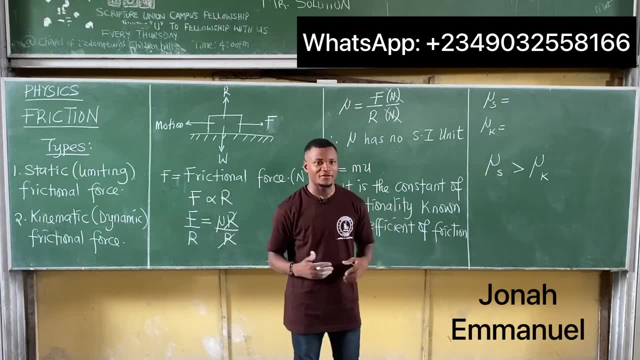 than I need to keep the body in uniform speed. we can now say that the coefficient of static friction is greater than the coefficient of kinematic friction. Alright, So with this, let's get some. Let's solve some examples and some vast questions. 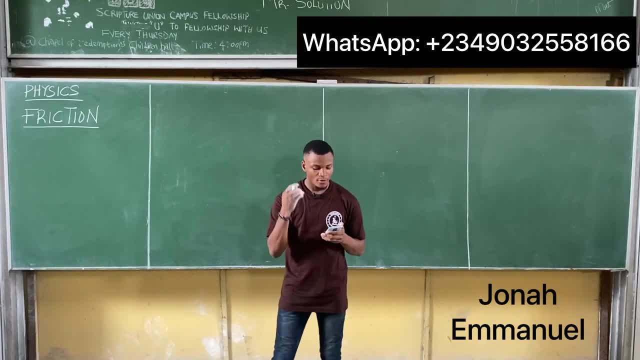 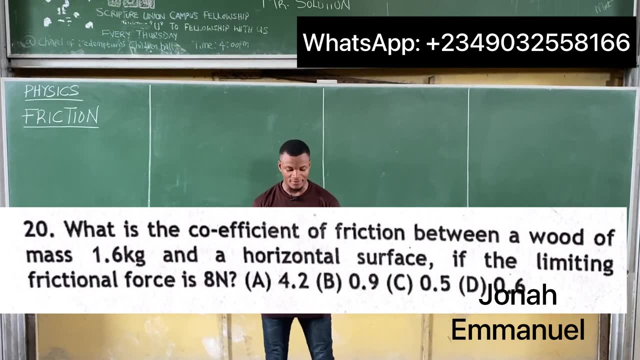 Okay, So let's take this sample problem. It says: what is the coefficient of friction between a move of max 1.6 kg and a horizontal surface if the limiting frictional force is 8 N? Alright, Let's get this done. 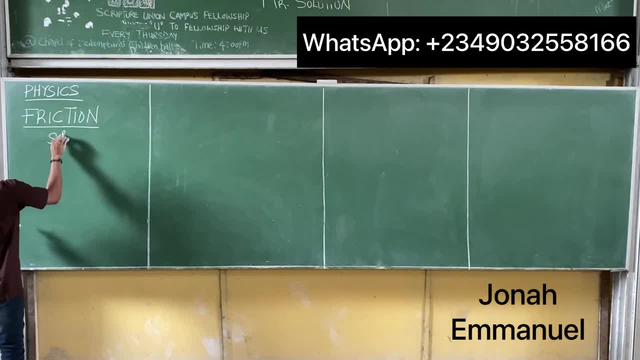 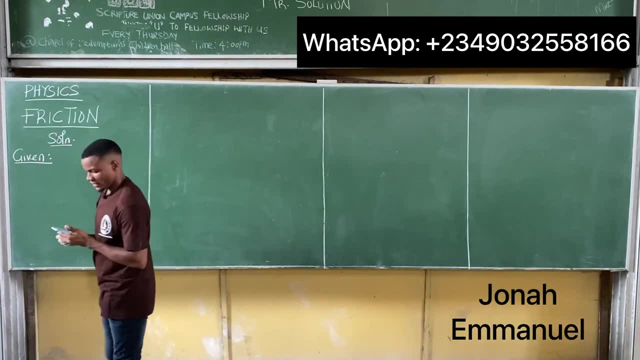 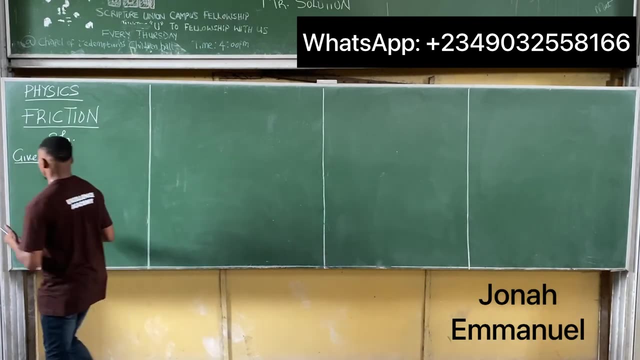 So solution: I will try to list out my given parameters So I can see what I have. So I want to say what is the coefficient of friction between a move of max 1.6 kg? The first thing that I'm giving number one. 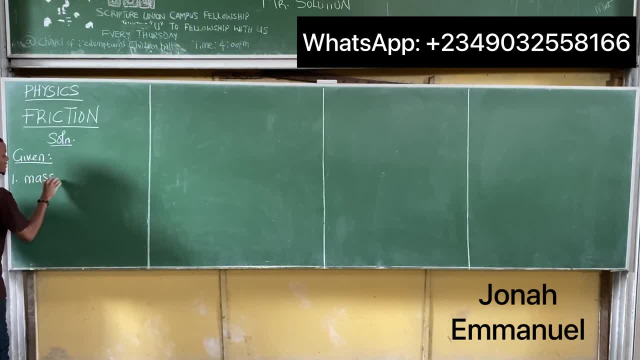 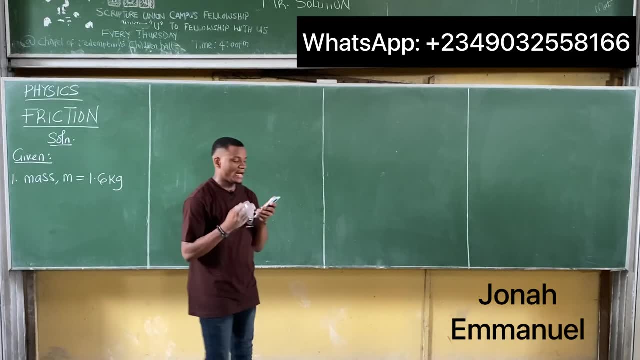 the first thing I'm giving is the mass of move. mass N is equal to 1.6 kg. So we have this Next what it says. and in horizontal surface, if the limiting frictional force is 8 N. 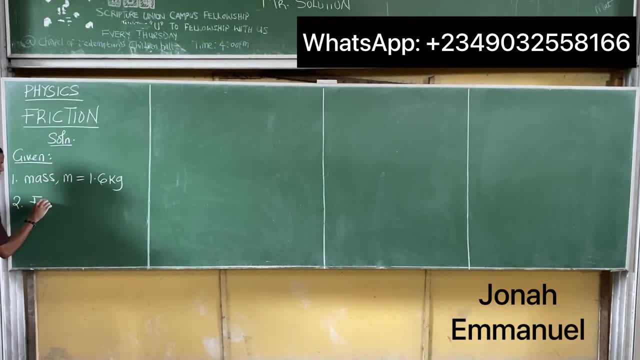 Number two: we have frictional force of perhaps limiting frictional force at 8 N. They said: what is the coefficient of friction? So number three: move. coefficient of friction is unknown. So let's solve this Now to get this done. 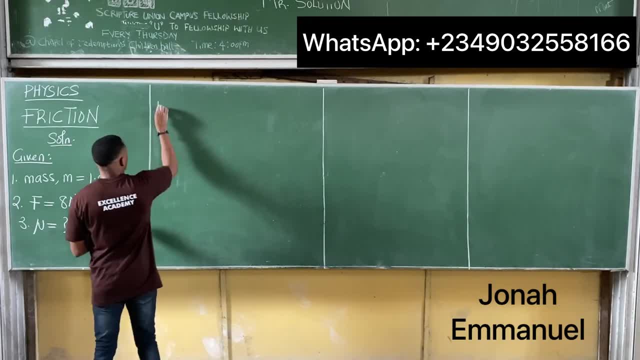 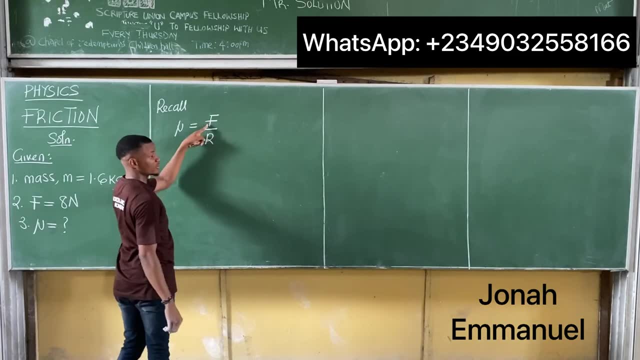 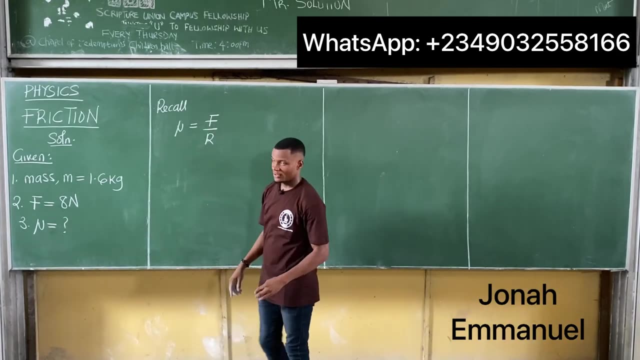 we have to recall our formula. Recall that we said: move is equal to F all over I, frictional force all over normal reaction. I already have the value for frictional force F, which we said is 8 N. My next task will be to calculate the value of normal reaction. 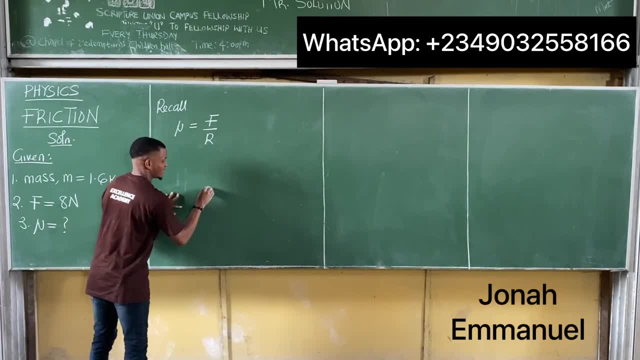 From my diagram I drew earlier. we said this: that for this particular scenario, I have weight acting upward and I have normal reaction. Sorry, I have weight acting downwards and I have normal reaction acting upwards. And we said that the normal reaction is equal to the weight of the body. 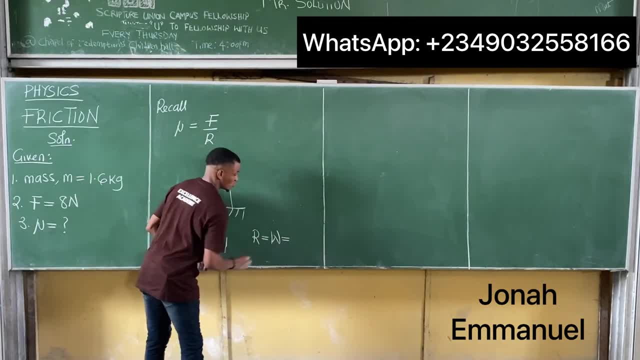 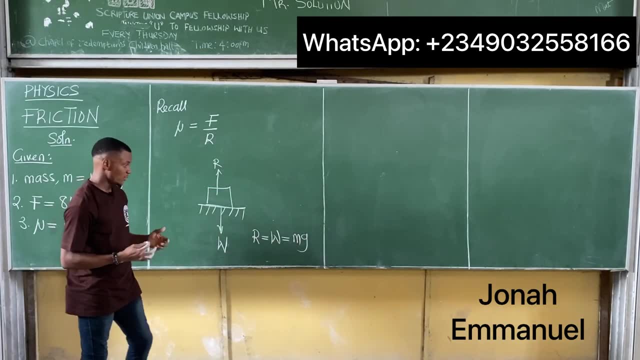 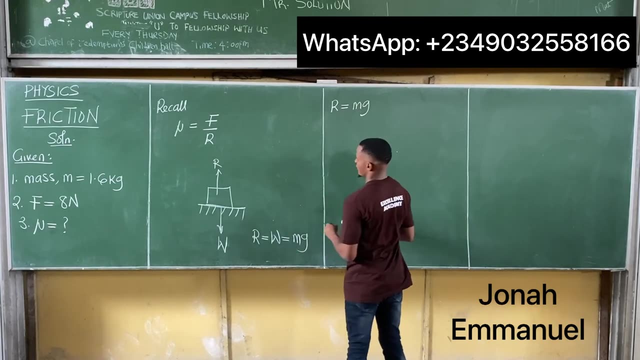 But also we know that weight is equal to the product of the mass of the body and acceleration due to gravity. So hence we can say that normal reaction is equal to mass times gravity. If I include this, the mass of the body is given by 1.6 times. 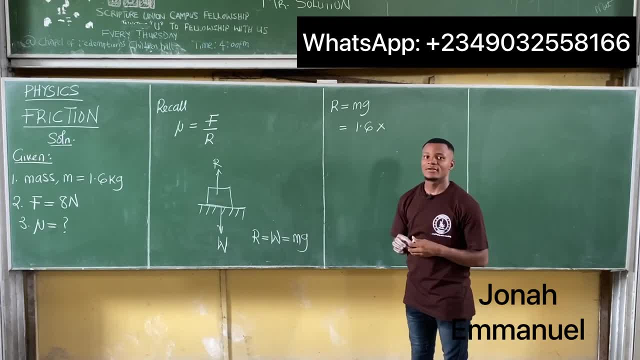 acceleration due to gravity is usually 10 m per second squared. Well, except you're given 9.8.. For this one, we have to give it as 10 m per second squared. If we multiply these two, we have that the value of normal reaction is equal to. 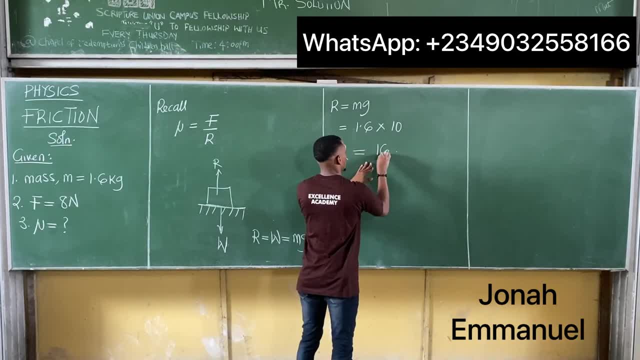 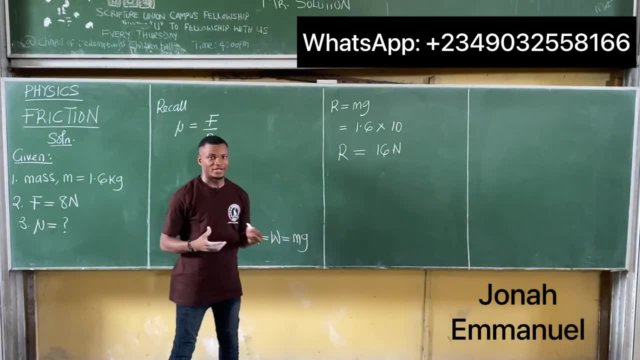 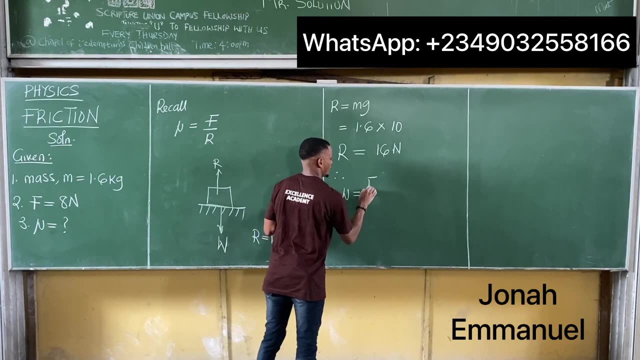 1.6 times 10, that equals 16.. Of course, 16 in Newton We said, normal reaction is measured in Newton. So therefore, therefore, the equation of friction is equal to F. all over I, That's equal to F. 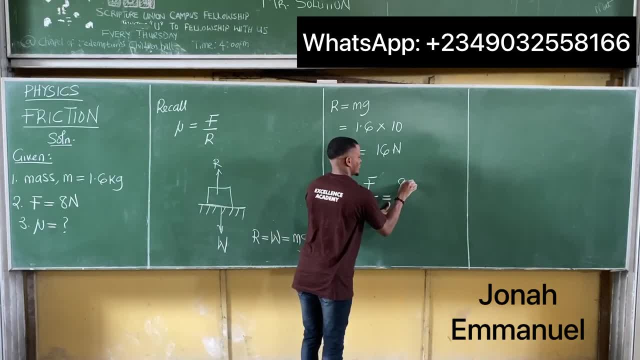 Frictional force, we said is 8 Newton, all over I. Normal reaction, we said is 16 Newton, All right. so if I open this, Newton cancels Newton 8 here, 1. 8 here. 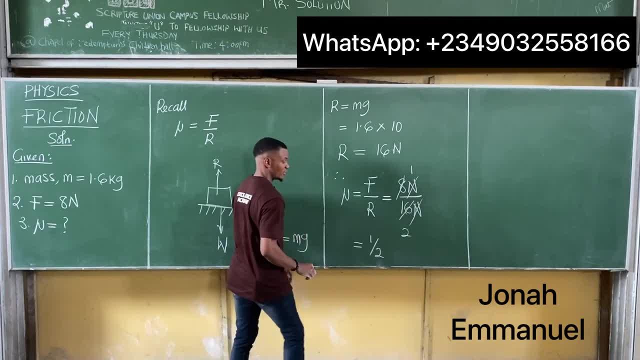 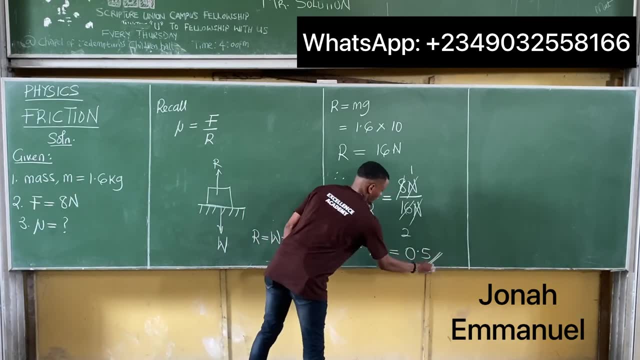 2. That's equal to 1 over 2.. In this example, that gives you 0.5.. So the coefficient of friction is 0.5.. Remember we said it has no SI, So the chance for this question. 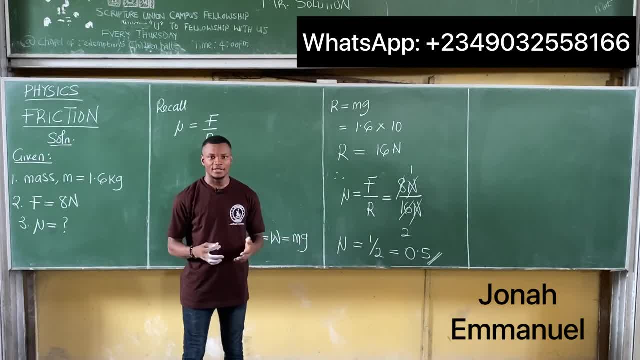 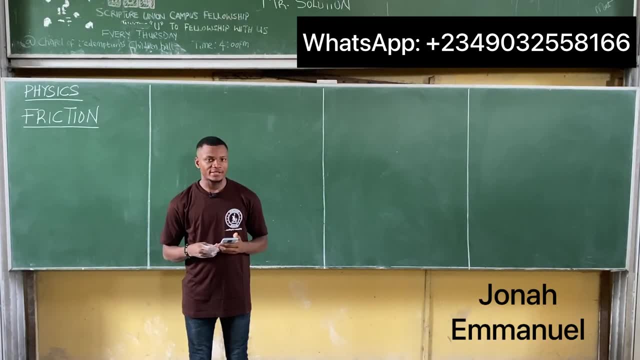 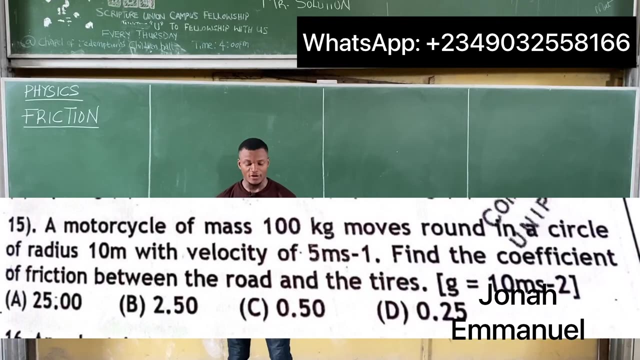 is 0.5.. This is how you solve this question. Let's look at yet another question on friction. Now it says a motorcycle of mass 100 kilogram moves at most ground in a circle of radius 10 meters with velocity of. 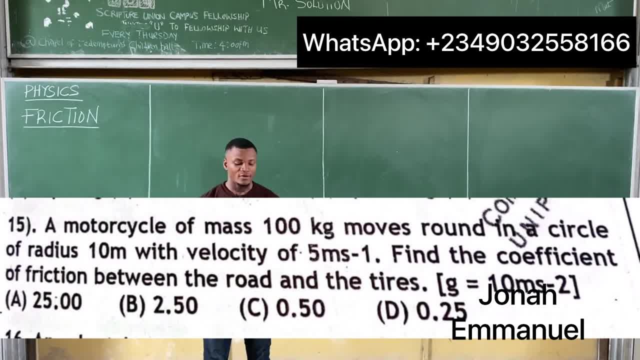 5 meters per second. Find the coefficient of friction between the road and the tires. Take gravity G as 10 meters per second squared. All right, so let's get this done. Solution: my task, as usual. first of all, 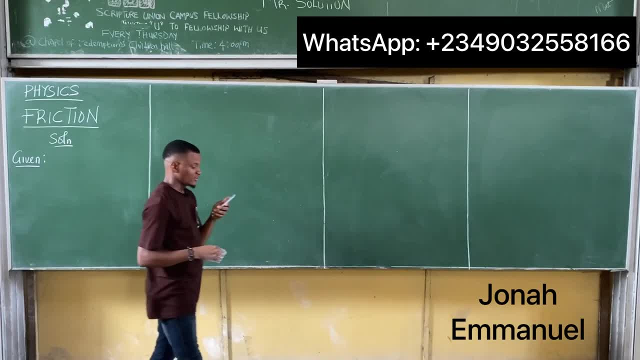 list out, given parameters. What am I giving? Like I said, a motorcycle of mass 10 kilogram by 1.. I'm giving the mass M as 10 kilogram. You see, moves ground in a circle of radius 10 meters. 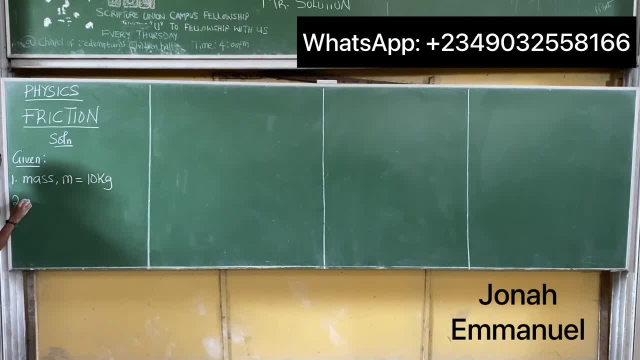 by 2.. I'm giving radius radius R as 10 meters. Next up a motorcycle with velocity of 5 meters per second. Number three, Number three: I'm giving velocity V as equal to 5 meters per second. All right. 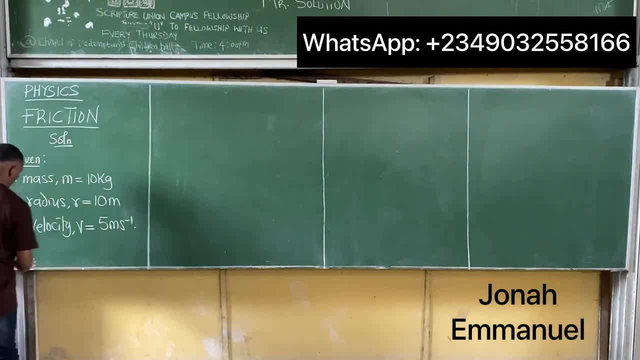 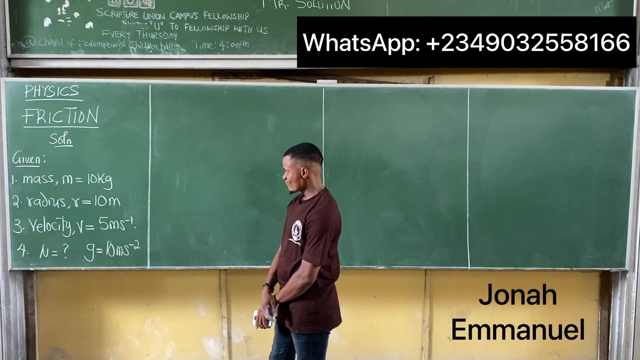 let's find the coefficient of friction. Number four: the coefficient of friction of move, is equal to unknown. G is 10 meters per second squared. So we have this All right. so you have to find, you have to find coefficient of friction. 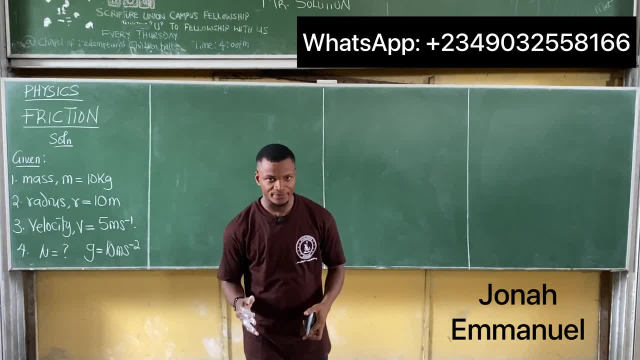 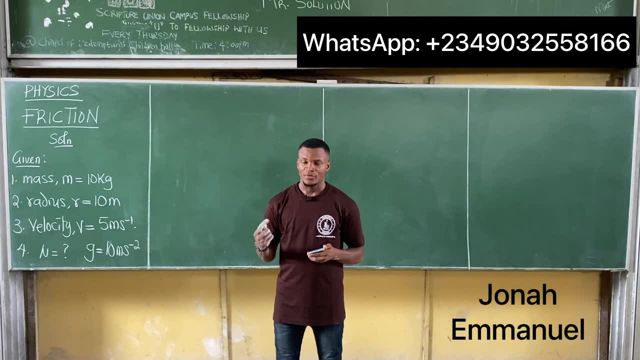 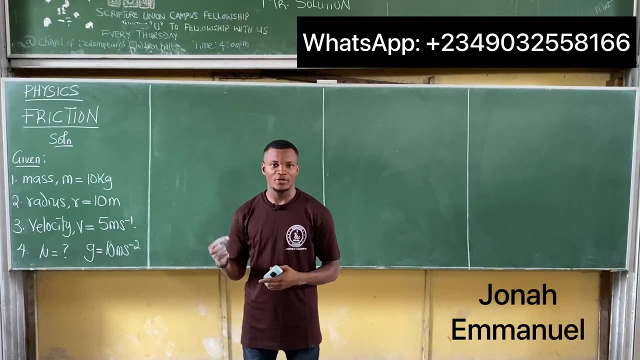 there. But here is a peculiar case. It's peculiar because this body is not just moving, but moving in a circular path. When a body is moving in a circular path, we say the particular force responsible for keeping a body moving in a circular path. 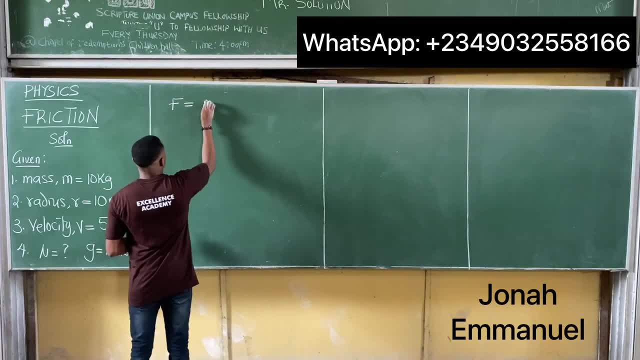 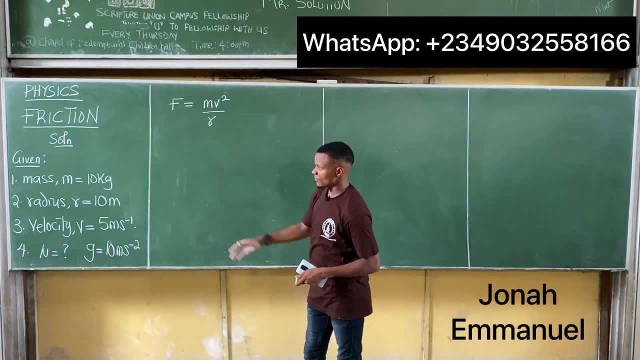 is called the centrifugal force, And centrifugal force F is given by m V squared all over R. All right, so the kind of force is m V squared over R. This is the formula for calculating the centrifugal force acting on the body. 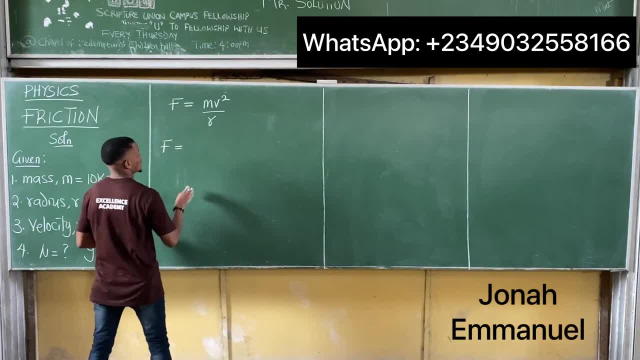 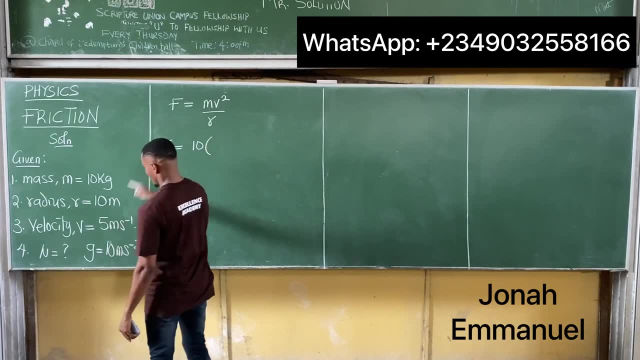 or causing the body to keep revolving in a circular path. If I include one here, you have the force. m is equal to m. that equals m in mass is 10 times V squared, So I have 10,. so I have this If I work on. 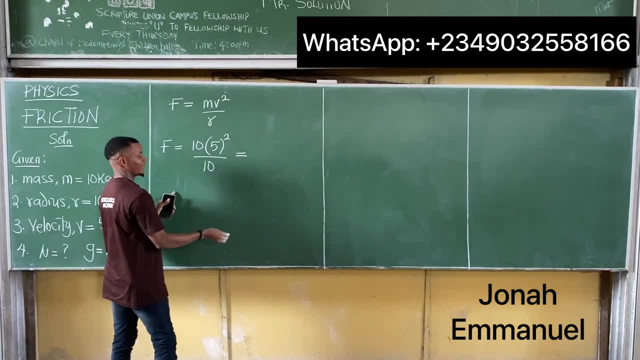 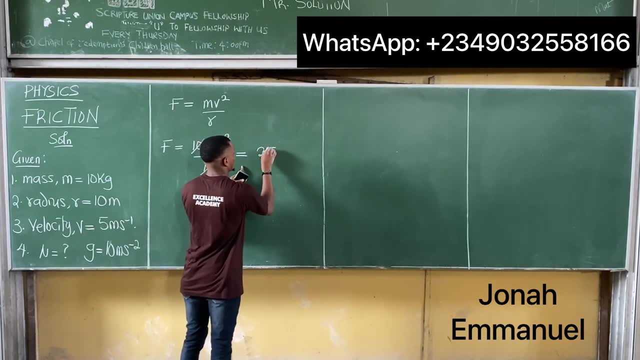 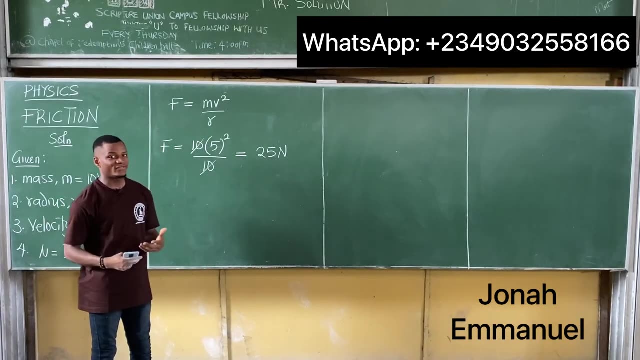 this. this is equal to an easy part. 10 can cancel 10, so F is equal to 5 squared. that equals 25 meters. So the centrifugal force in this case equals 25 meters. Now I'm repeating the circular. 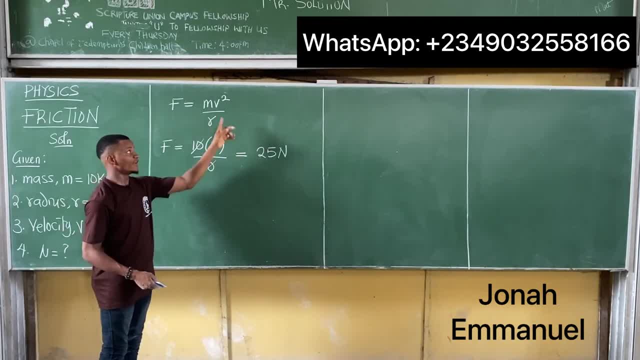 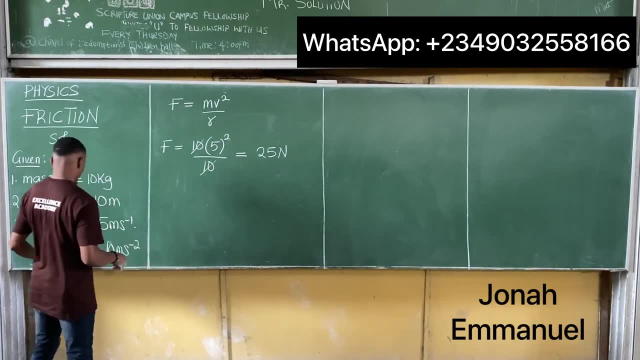 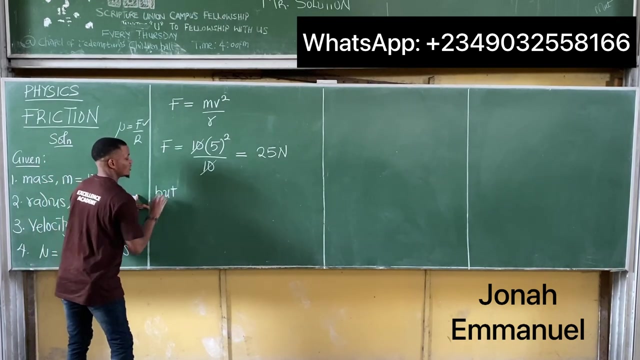 path And for centrifugal force, the force is equal to mass squared all over radius of path. That's it. Next I'm going to. we have to find coefficient of friction. We look at the coefficient of friction: move is equal to F. 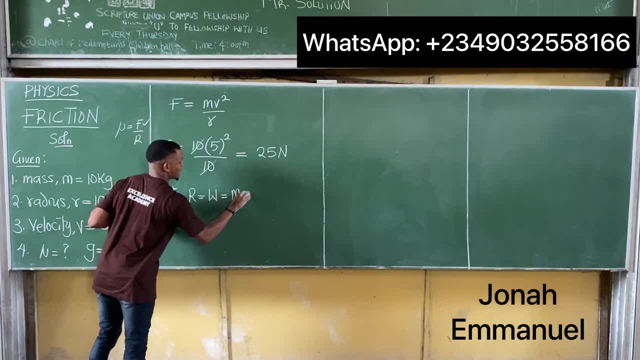 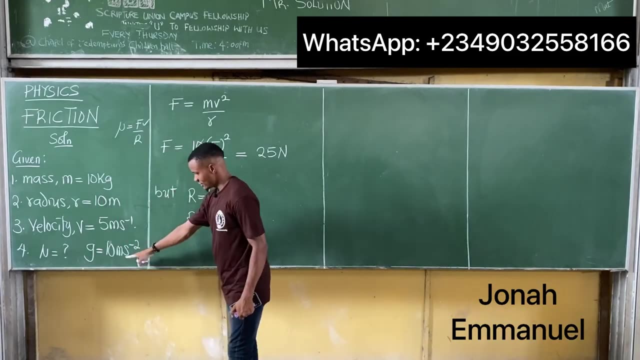 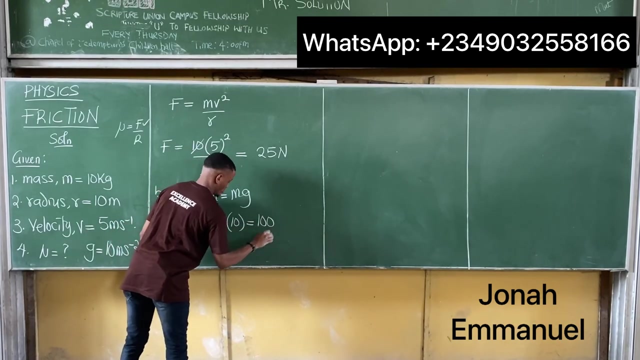 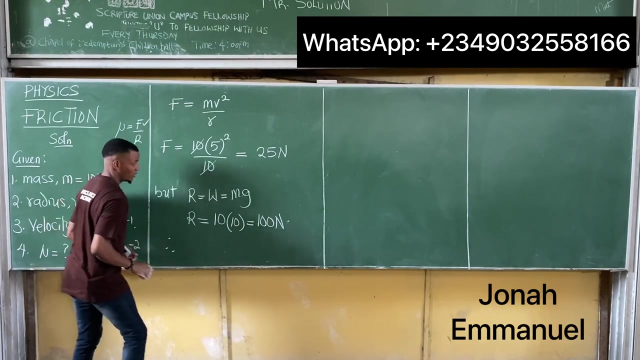 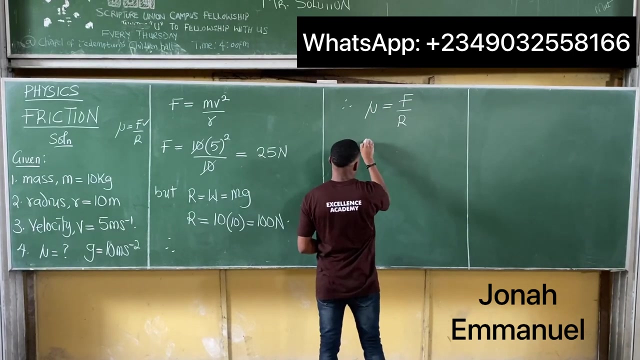 all over radius of path. Now, what is the mass of the нек term? This is the constant mass of gravity, exactly the mass mass of gravity. And this equation is also equal to. So therefore say: mu is equal to F all over I. that's equal to F. frictional force: F is 25,, that's 25, all over I. normal reaction is 100. 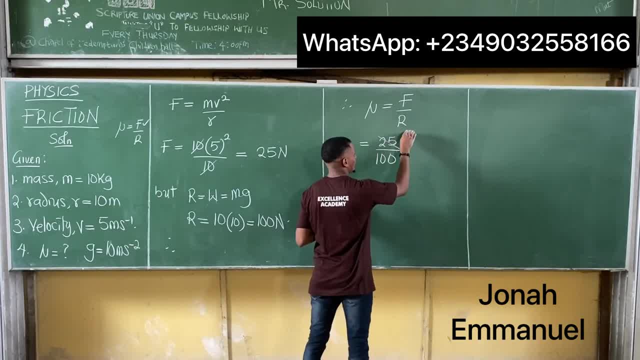 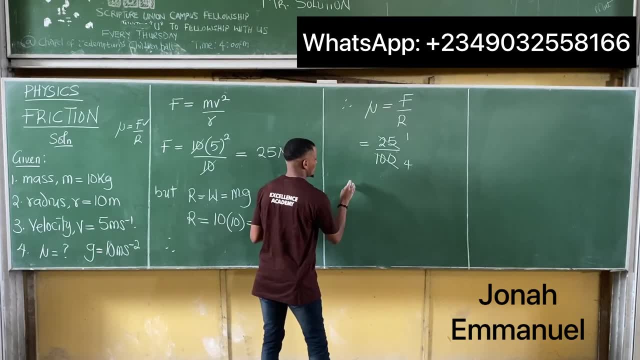 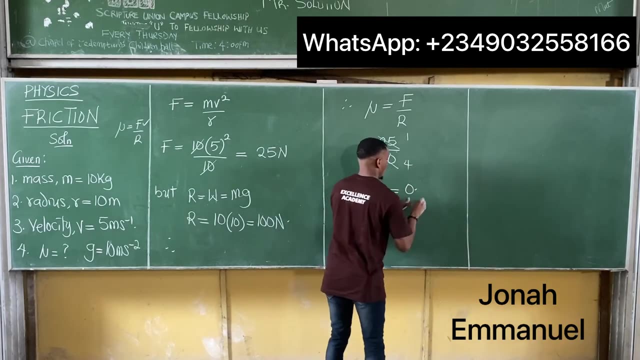 If I work this out here, 25 has itself 1,, 25 here I have 4, so the frictional force, or sorry, the normal reaction mu is equal to 1 all over 4, which in decimal gives you 0.25. 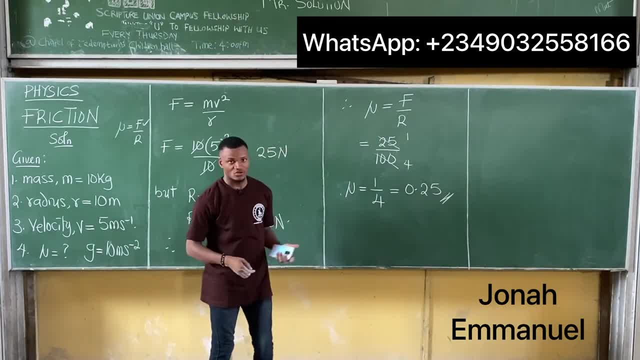 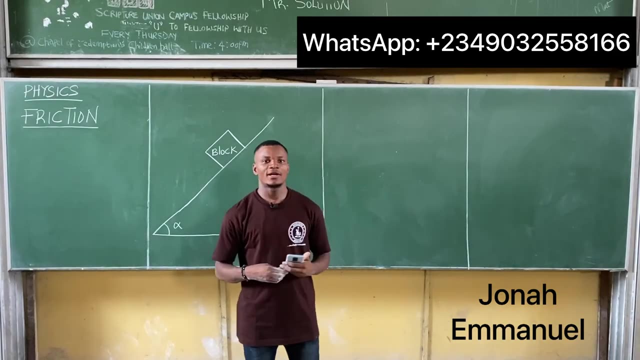 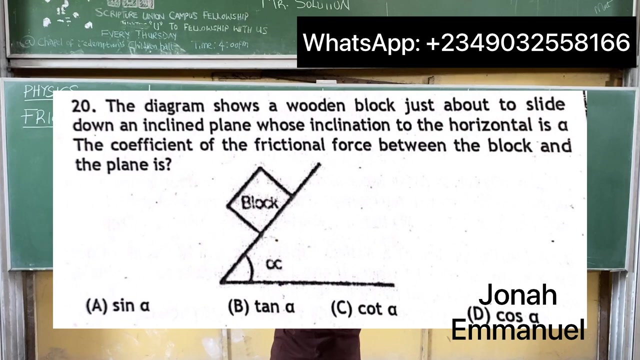 Of course there is no S in it. so mu is equal to 0.25, and that's your answer. Alright, so this is how you solve this particular problem. Let's consider one last example on that friction. The example says: the diagram shows a wooden block just about to slide down an inclined plane whose inclination to the horizontal is alpha. 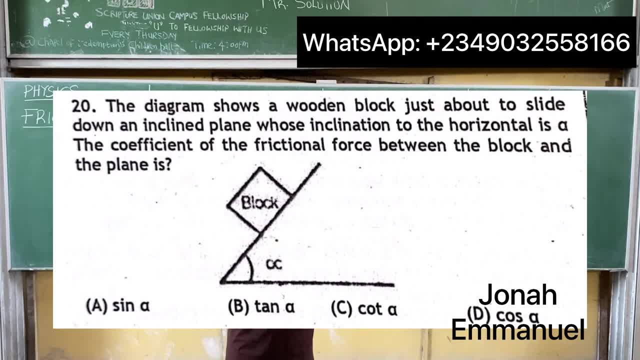 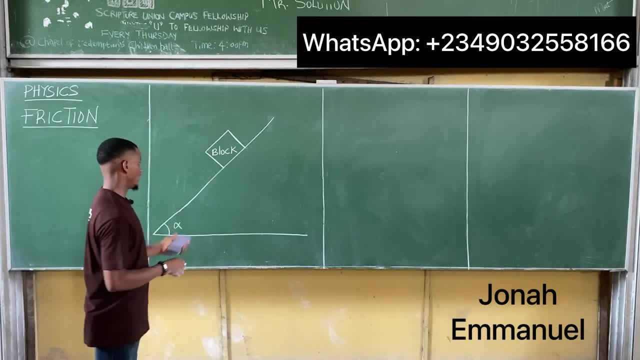 The coefficient of the frictional force between the block and the plane is. so you have your options there. Alright, let's get this going. So we have this as a case. we ask to find the coefficient of friction in this case. what do we do? 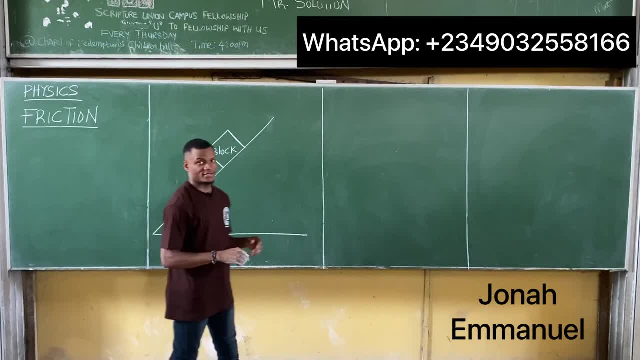 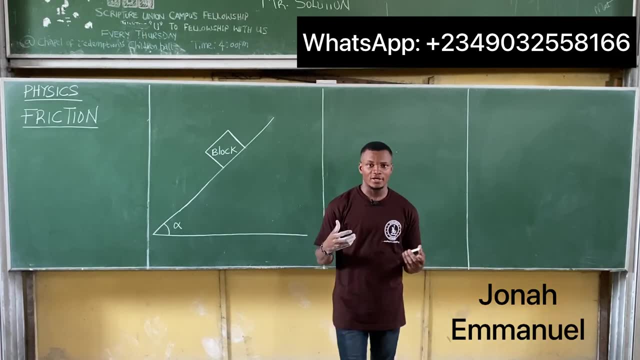 Now, first things first. this is an inclined plane. we've already dealt with inclined planes in a previous video. I'll leave a link to the video on inclined planes in the description of this video, Alright, so at this point here, let's deal with this. 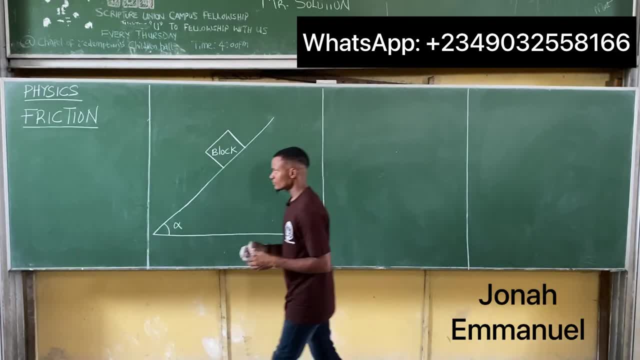 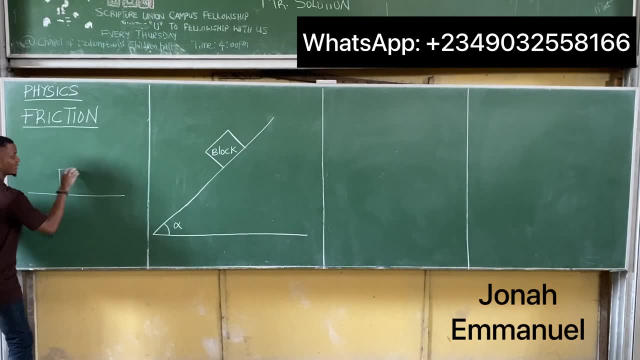 Alright. so at this point here, let's deal with this. Alright, so at this point here, let's deal with this. So first things first. here's what we know. We said, when a body is placed on a surface, as in this case, that what acts here is called a weight, what acts here is called normal reaction, or here they call it a block. 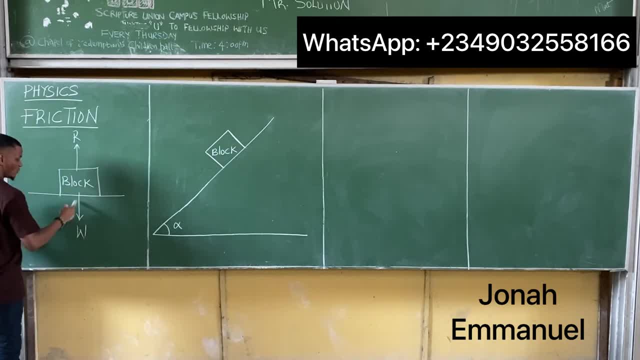 So perhaps let's say: when a block is placed, weight acts this way, reaction acts this way. we said, if this is the motion of the body, here is the reaction, Here is the reaction. It is displayed is with the friction of the body. 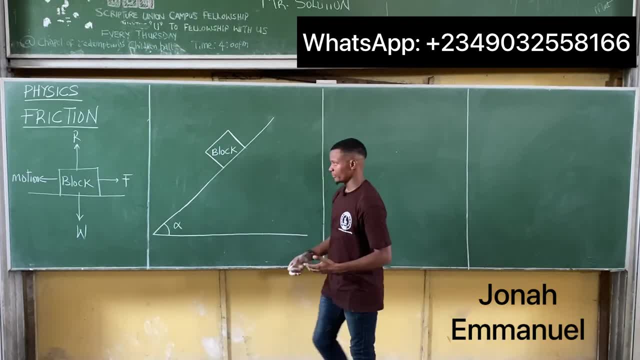 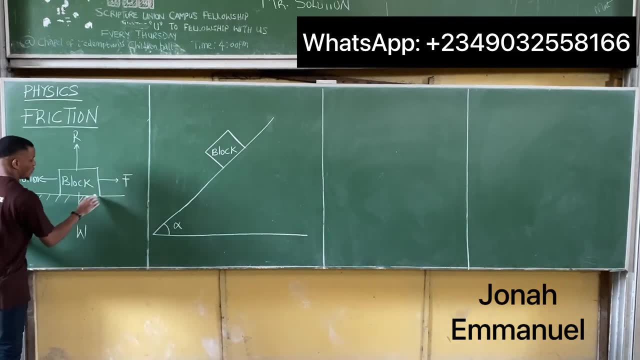 So they established this fact in a previous conversation. So they established this fact in a previous conversation, So let's use this idea here. What if this is no longer a rough surface like this? What if this is not an inclined plane? Now, here's what we know. 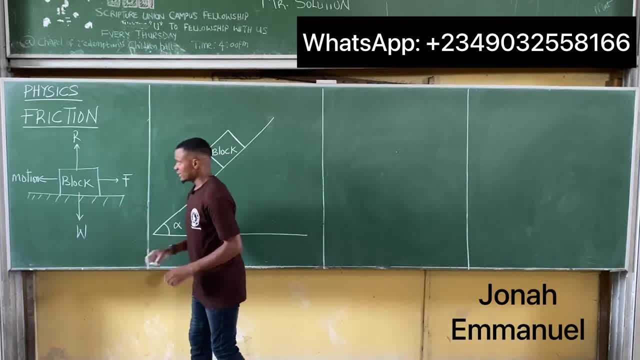 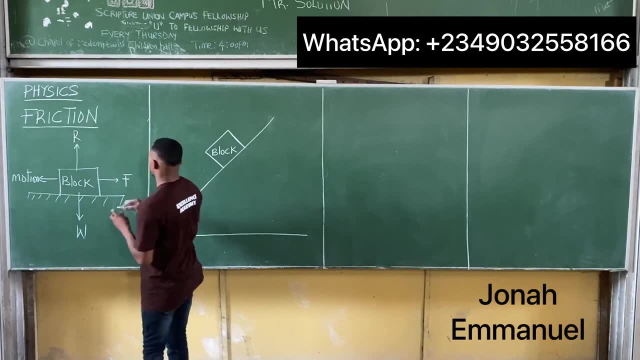 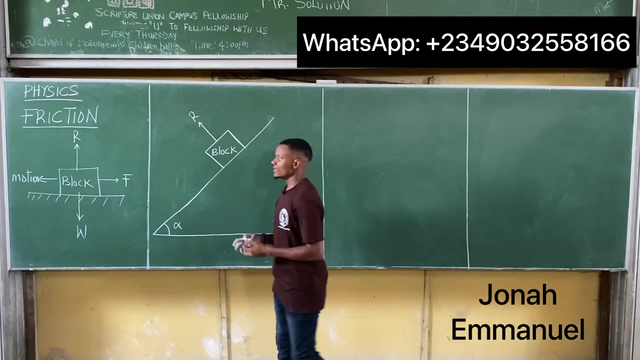 Number one: weight acts in this way. Now, if I look at this correctly, normal reaction acts upward. So upward, here should be normal reactions that are additionally pulsating. So upward, here should be normal reactions that are Gesundheit, and this is normal reaction, and that's number one. next up, you would assume that normal reaction and 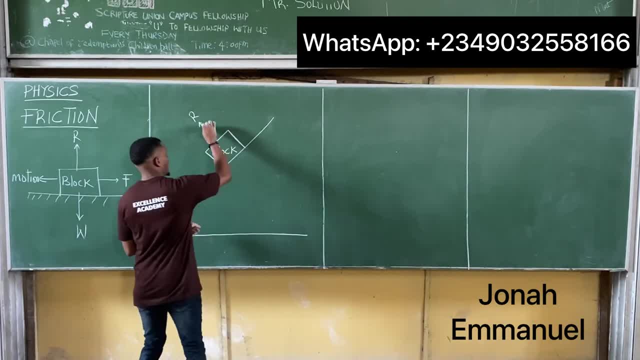 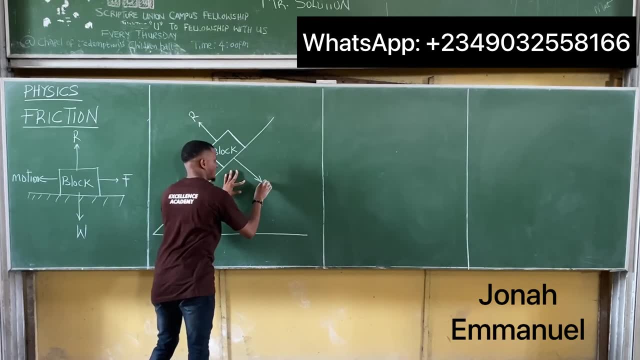 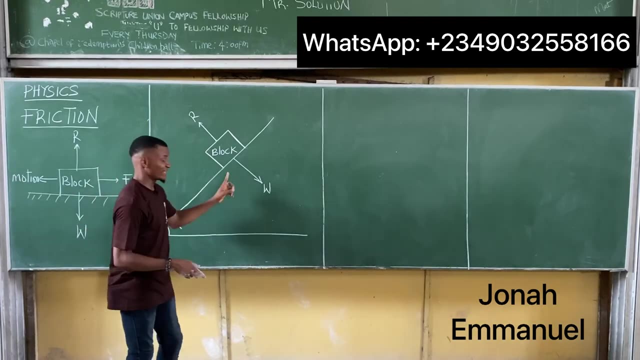 weight are in a straight line. that means, from here i should have taken a straight line this way. i should have my weight acting this way, that's weight acting this way- done. this is what we should have, this is what we should expect from this diagram, but in reality, this is not so. 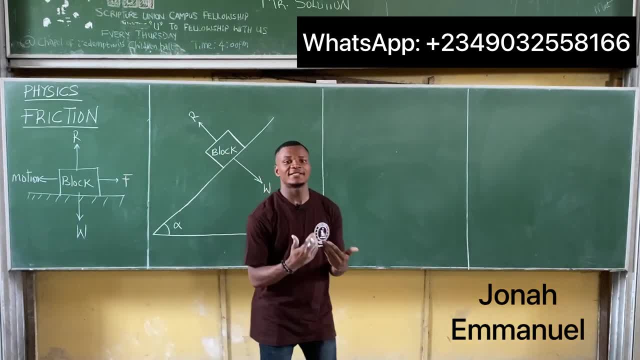 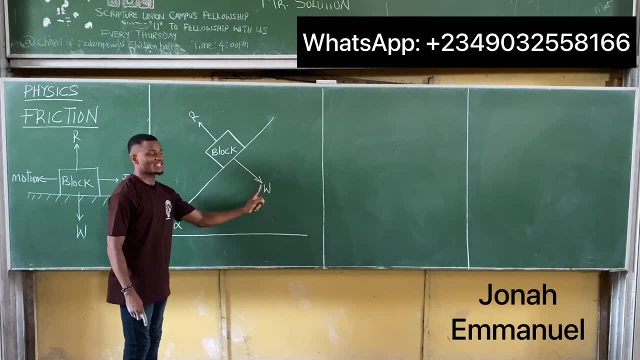 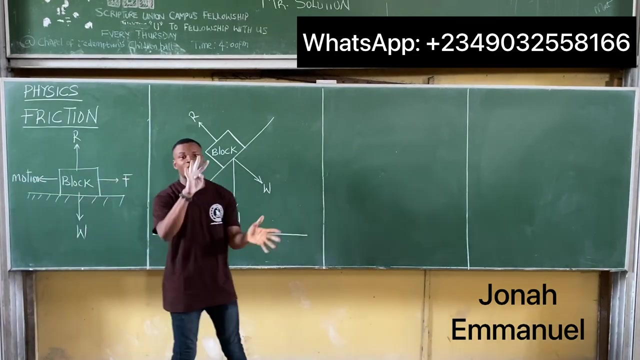 the idea is this weight always acts vertically downwards. so in this case, here, your weight cannot act this way. this, this idea of weight acting this way, is not practical in a practical sense. the weight will not act this way. it must be vertically downward. so the weight must always act vertically downward, irrespective of how you place the body. 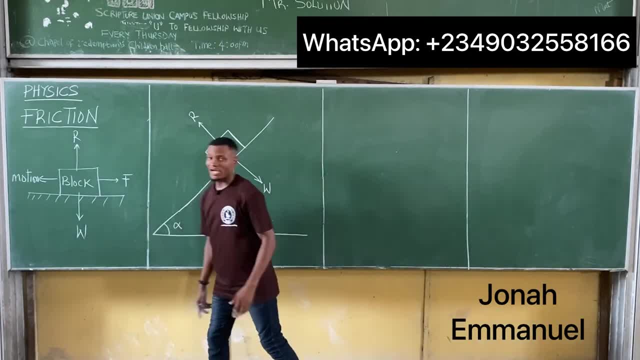 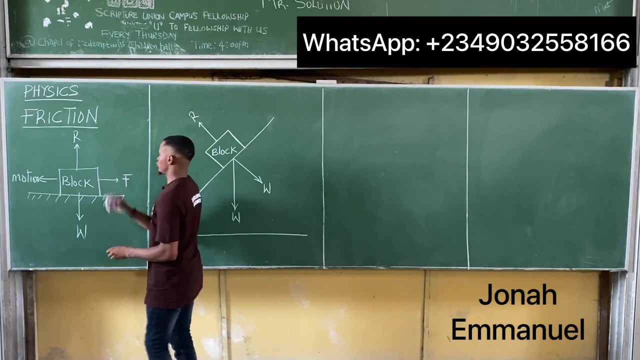 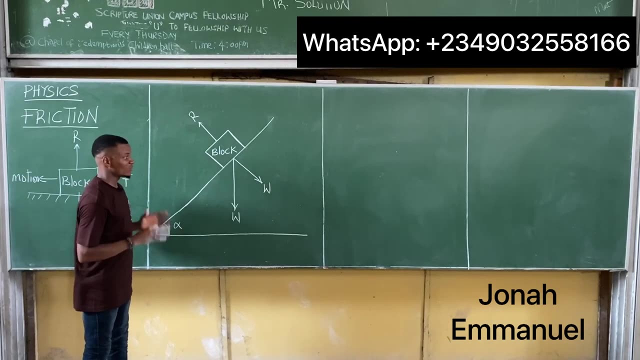 the weight will always act vertically downwards. but then this should be my hypotectical weight, this one here. what i'm seeing, opposite, the normal reaction. if that is so, we have to do a little bit of analysis, and by analysis you have this: if a body is inclined on angle alpha to an inclined plane, 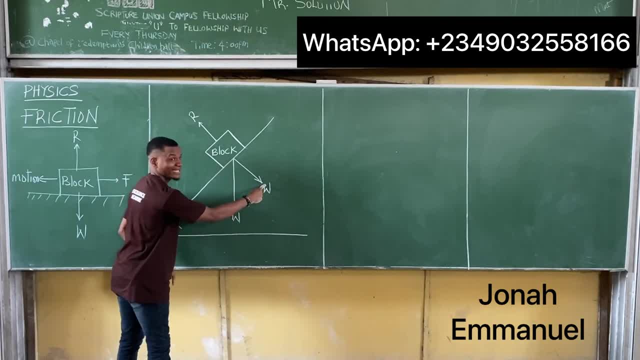 the angle between the hypotectical weight- that's what here- and the view with this angle here will be the same thing as this angle here. so, yes, still becomes alpha. So we have this. So hence you can see that the weight is inclined at an angle alpha to the vertical. 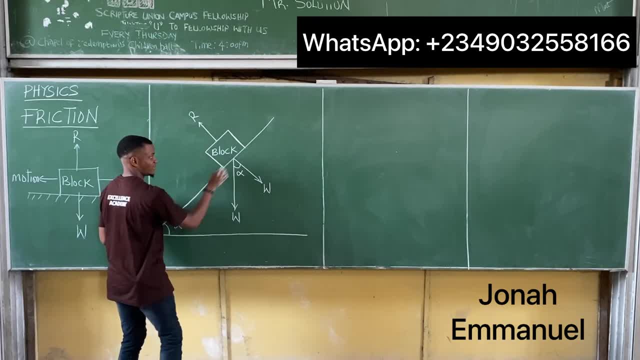 That's again the weight. So you might have this: This becomes my horizontal line, This becomes my vertical line This way. So I'll just call this a V. This is V. V means vertical line, H is horizontal, So it was just this. 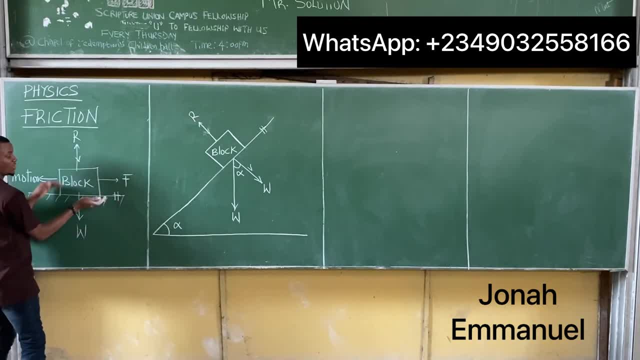 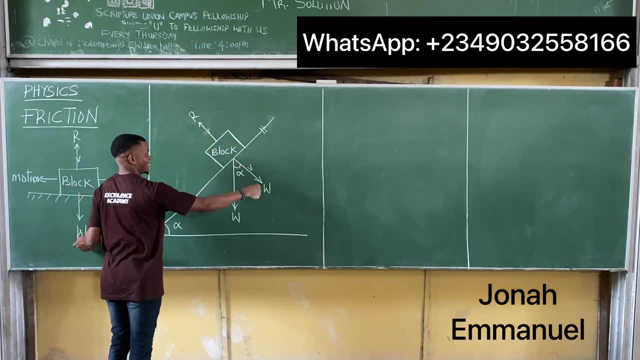 So this is my horizontal, This is my vertical. It was just slanting like this And I have this. This is still the horizontal, That's this. And this is still the vertical. That's this, Alright. So in this case, here's what you note When a force or when a vector is inclined at an angle theta, or, in this case, alpha- to the vertical. 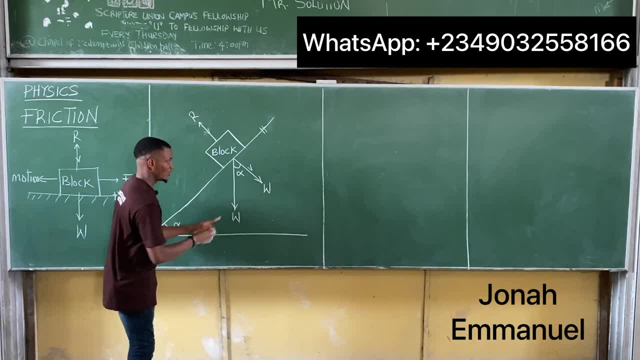 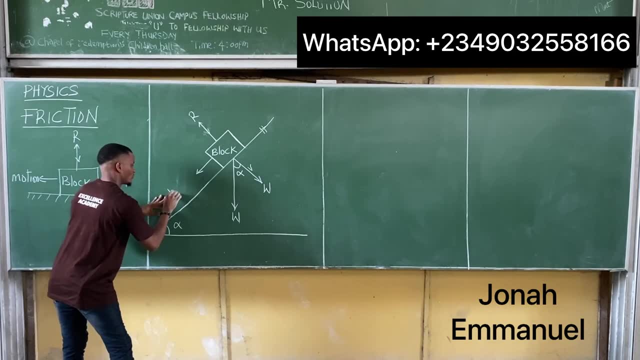 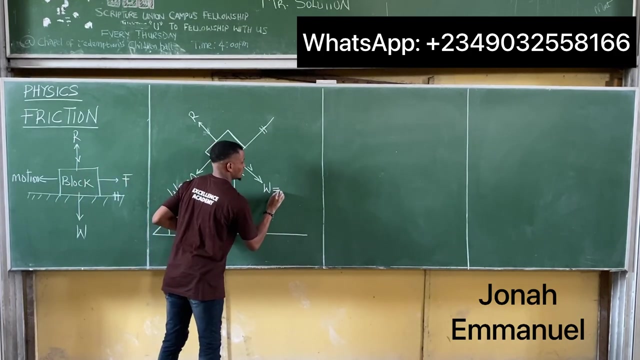 the horizontal component of this vector, that's the one that acts here, is given by this W, this one here is this sine theta. That is this part here. Alright, While the vector component is given by W is equal to: this is equal to W cos theta. 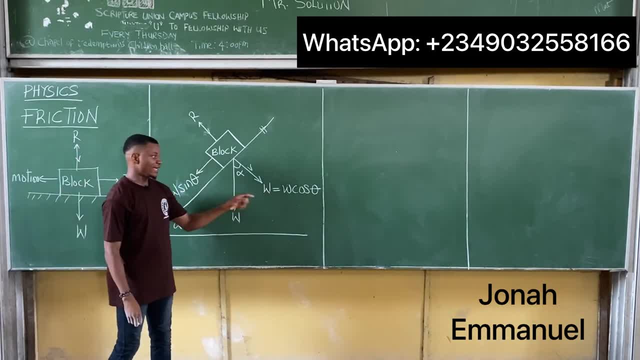 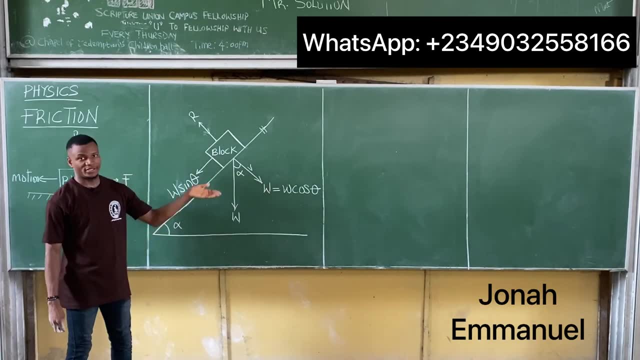 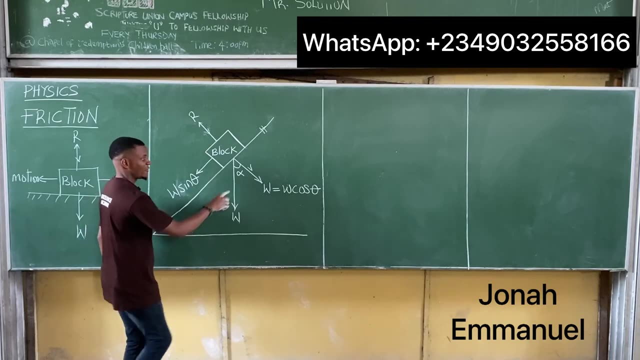 What we are having W sine theta and cos theta is because we are resolving this Both, Both horizontally and vertically. So this one has already been explained in another video. So just note that if a body is inclined at an angle- sorry, we are using alpha here- 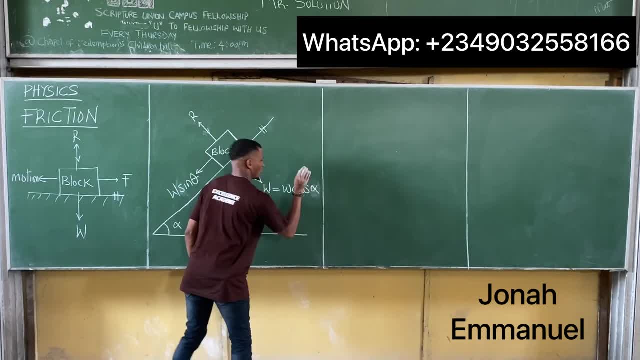 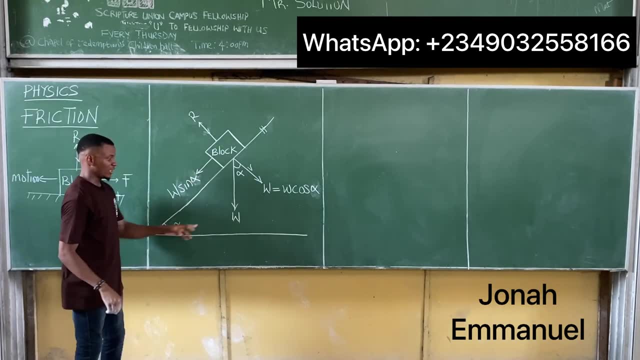 So next, let's use alpha instead. Cos, alpha, cos of an angle. Can you hear it? Cos, alpha, cos of an angle. So if a body or if a force or a weight or any other vector is inclined at an angle alpha to the vertical. 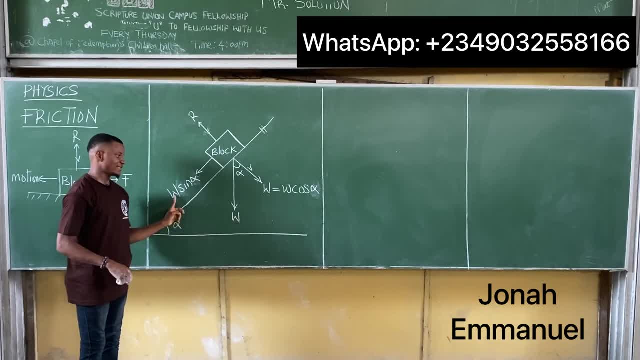 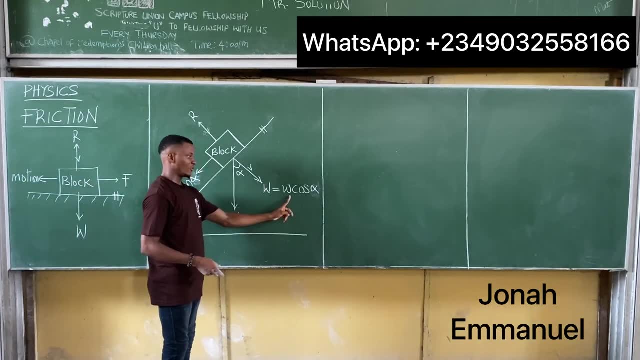 the horizontal component becomes this: that that vector, in this case weight sine of the angle, and the vertical component becomes that vector, cos of alpha. Alright, After we have established this, we can see that R is equal to this one here. 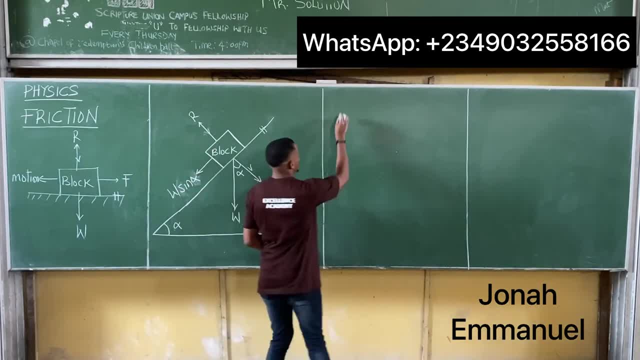 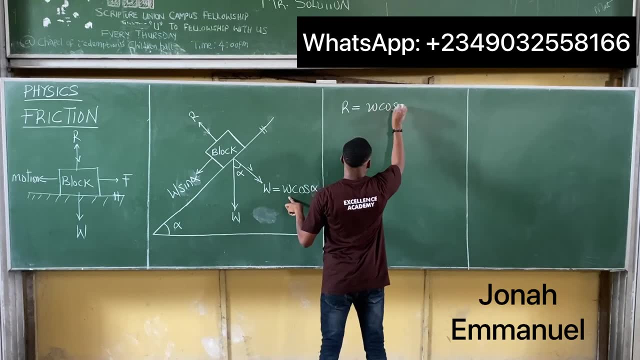 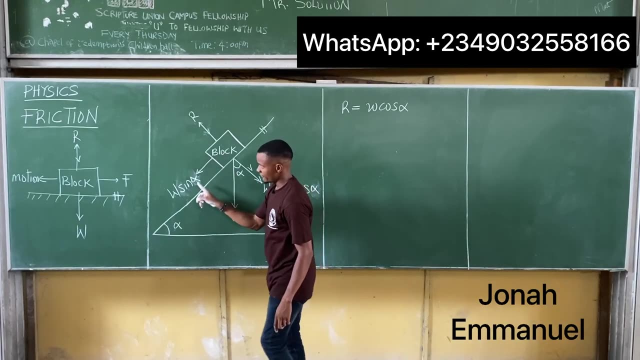 So R is equal to. from here we can see that R is equal to this. one is equal to this one here: W cos alpha. So we have this While this one here. for this, if I compare this to this one here: 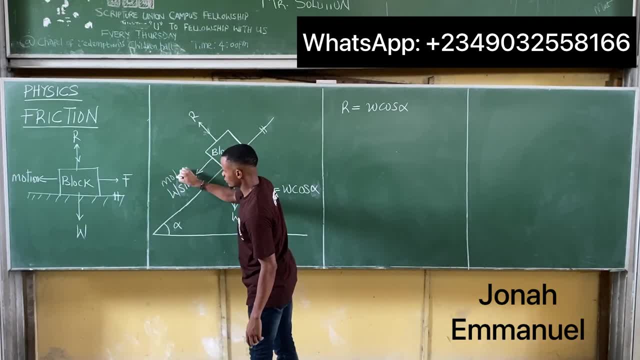 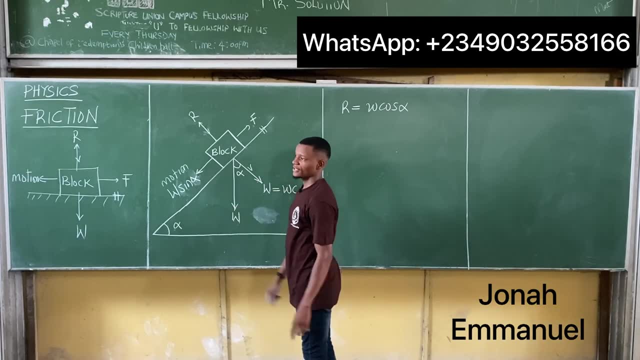 of course this one will slide here. This becomes the motion. It will slide here. Frictional force will act this way, trying to oppose this block from sliding down, And the frictional force F is equal to the motion. that's W cos alpha. 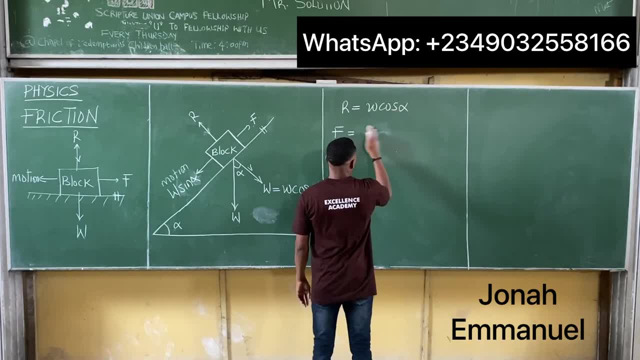 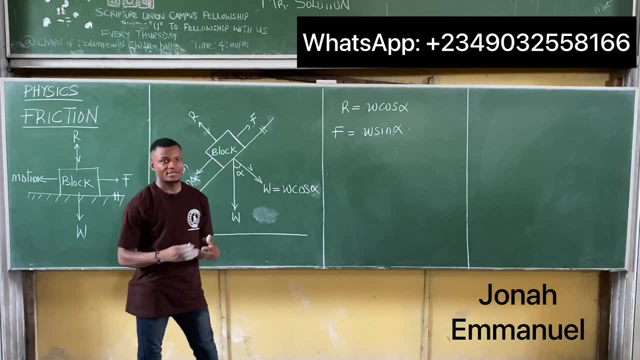 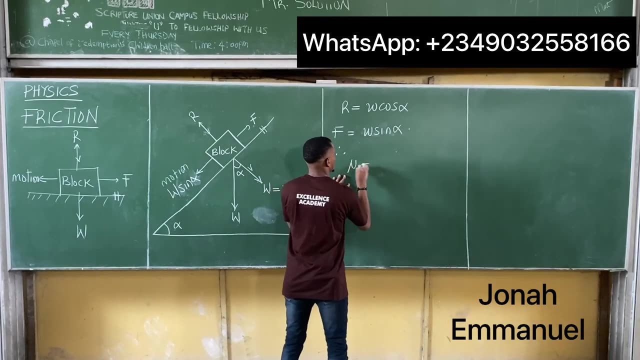 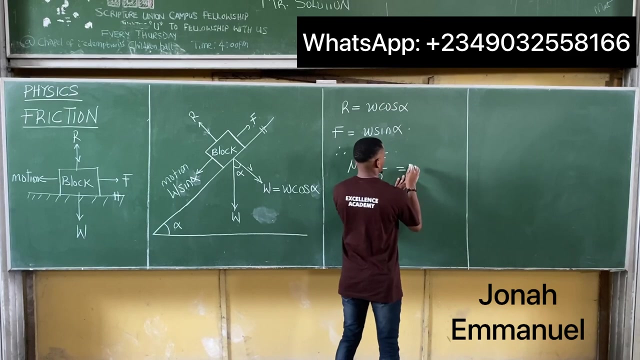 That's W sin, that's W sin alpha. So we have these two identities. So therefore the co-equivalent friction, this move, which is equal to F all over R, when that's equal to F, is W sin alpha all over R. 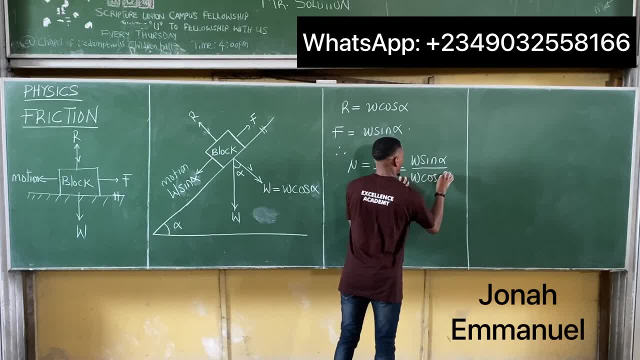 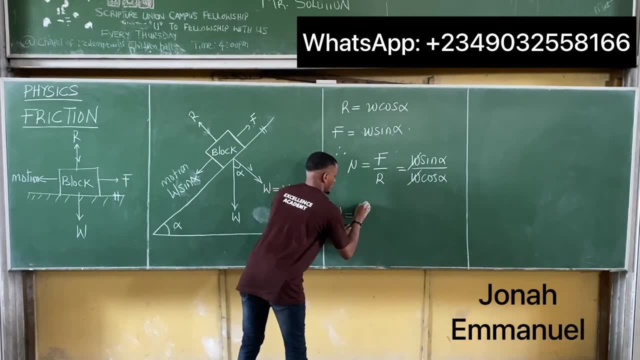 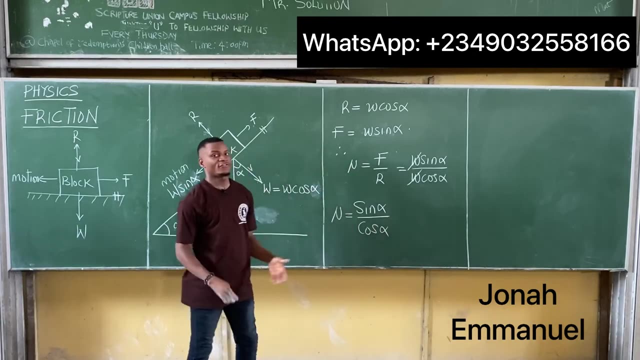 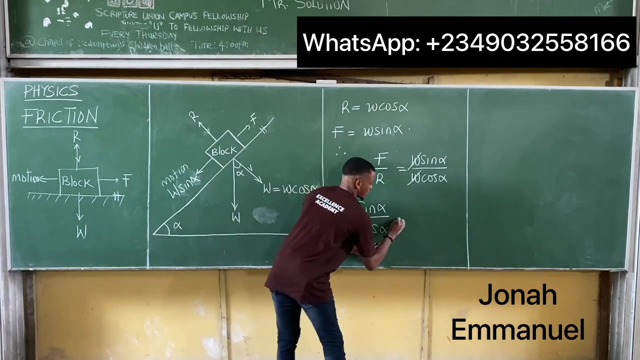 R is W cos alpha. From here, W cancels out. So co-equivalent friction is equal to sin alpha all over cos alpha. And if you're coming down with three, that's two metric identities. We said: sin alpha over cos alpha gives you tan alpha. 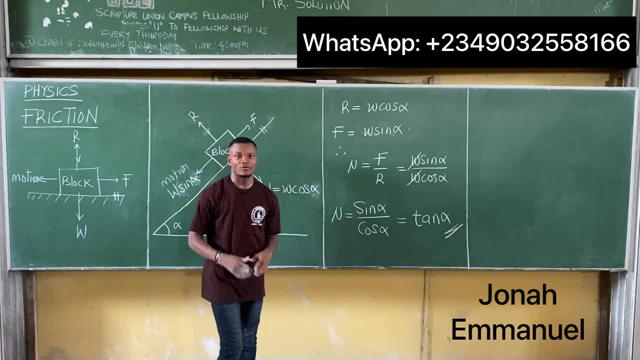 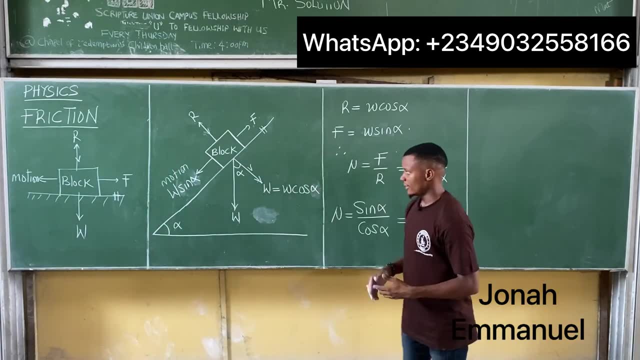 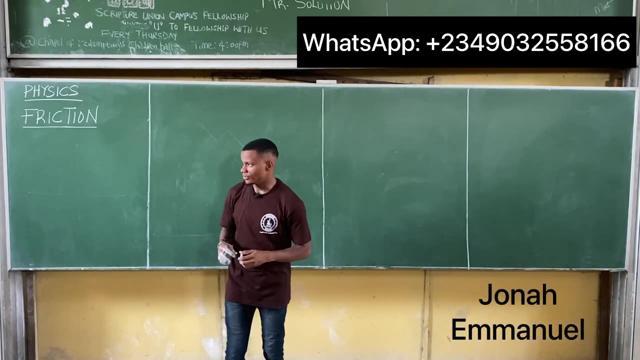 Alright, So this becomes your answer. Hence, the answer to that question is tan alpha. So this is how you solve this particular question. So we'll end by looking at some of the advantages, disadvantages and some ways in which we can reduce friction. 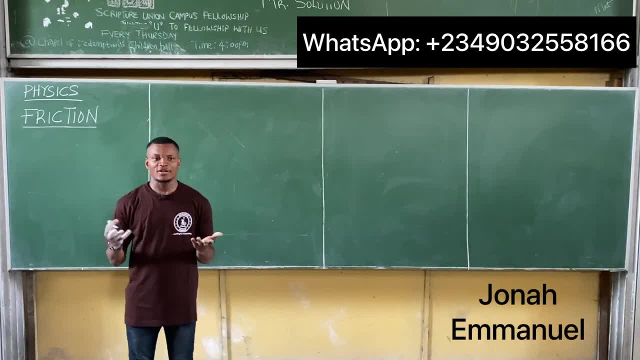 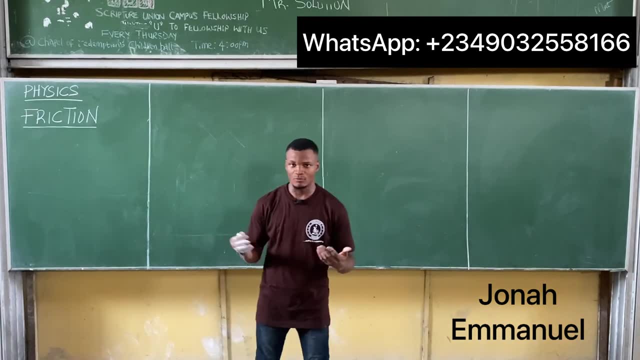 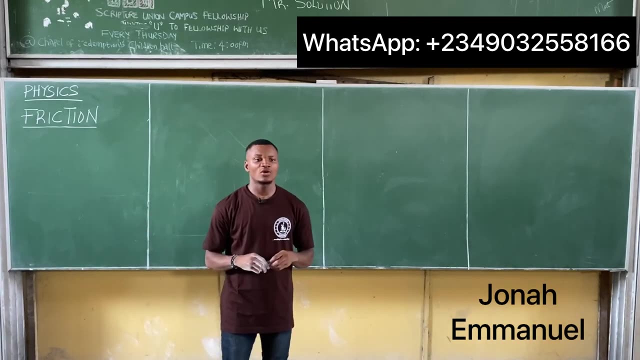 Let's start with the advantages. Some of the advantages of friction is that friction helps us to walk, to run, to jump, So I can actually stand here or I can move around here because there's friction between my toe and the ground. Friction also helps us in wrapping things. 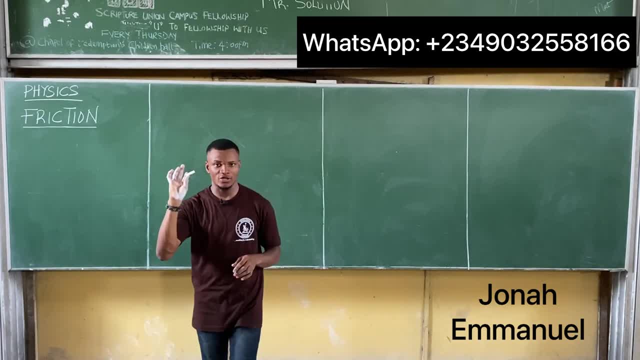 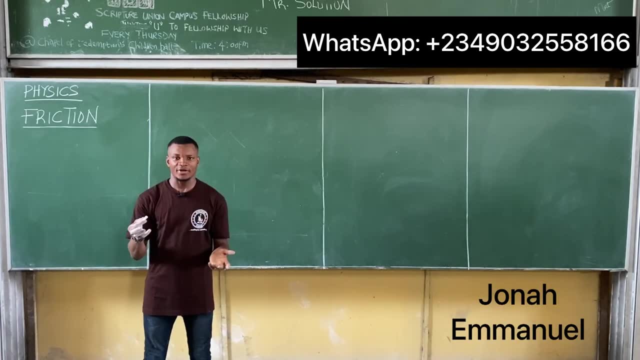 You see, why I can hold this piece of chalk is because a frictional force exists between the chalk and my hand. If the chalk is too slippery, what you observe is that it falls off of my hand and I can't hold it. In fact, this explains the reason why I can't hold it. 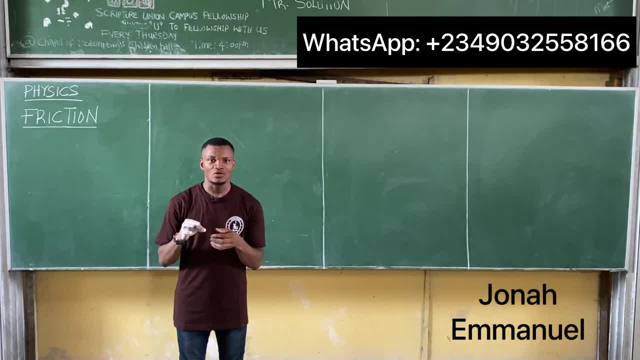 Friction also explains the reason why you cannot hold slippery objects. So why is that Whenever you hold a slippery object, it just falls from your hand? Or perhaps if you step on a slippery ground, or perhaps a wet tarp, for example? 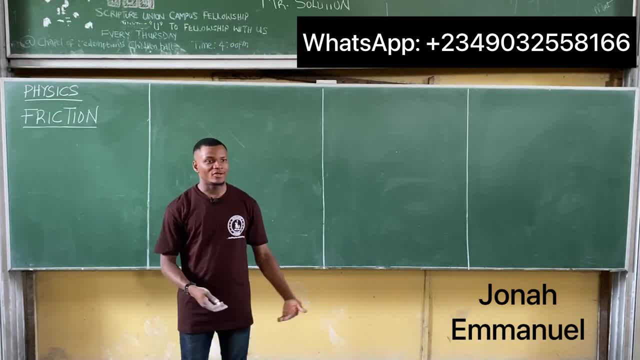 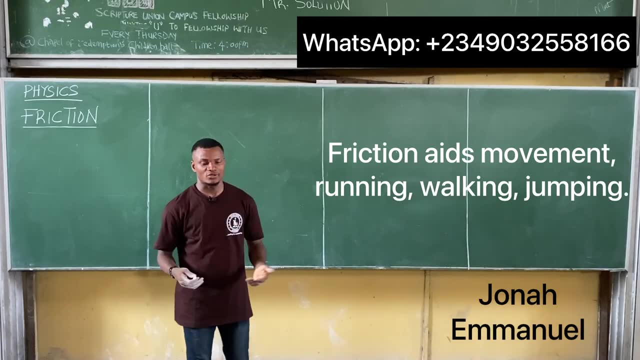 a tarp that is wet, you slip and fall. Why? Because there's little or less friction there. Alright, So the advantages are: number one: friction helps us to run, to jump, to walk around. Number two: Friction helps us in grabbing things like this. 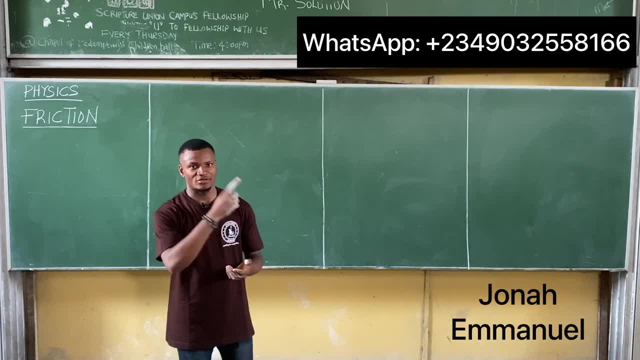 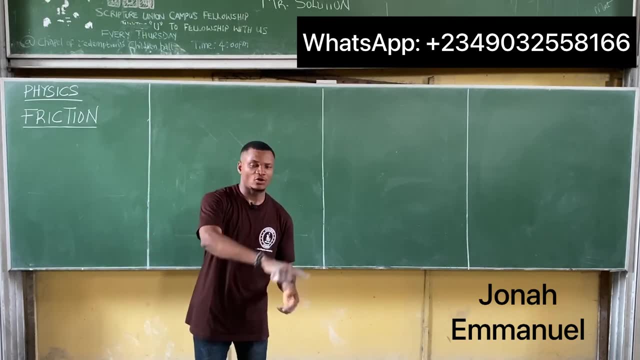 Number three is that friction also helps in belts to drive Alright. In the case of pulleys, where you have belts or pulleys, the reason why those belts can actually connect to those pulleys is because there's friction existing between them. So these are some of the examples or the advantages of friction. 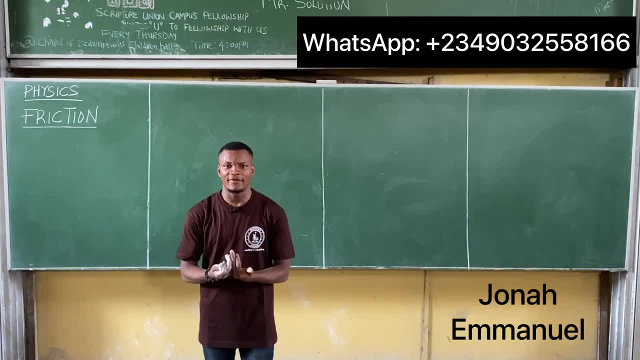 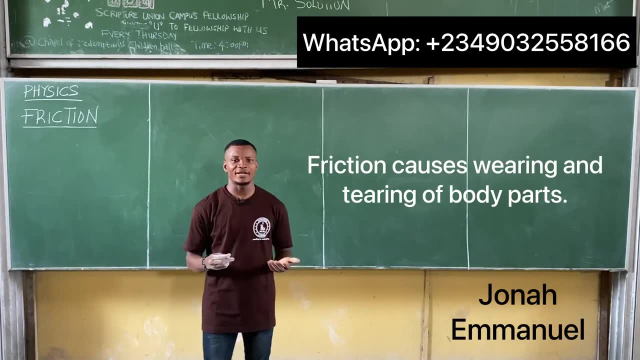 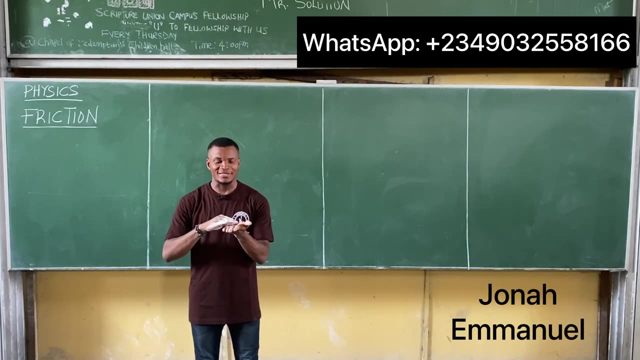 So, aside these advantages, what disadvantage or disadvantages does friction possess? Number one: Friction causes wearing and tearing, And this is why you have to change your car tire regularly. Alright, It becomes slimmer in quotes as you use them. 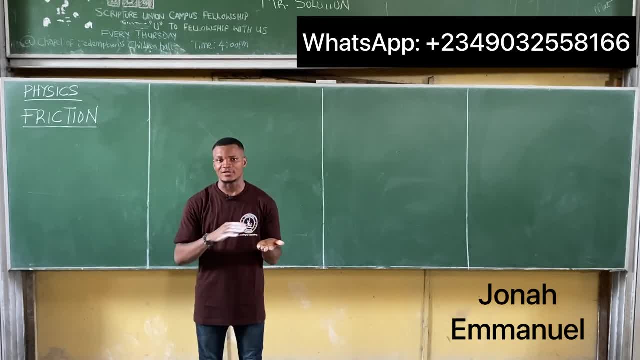 Why? Because the surfaces of objects wear off due to friction. Okay, When they rub against each other, they wear off. That's number one. So the first disadvantage is that friction causes wearing and tearing. That's number one. Number two: 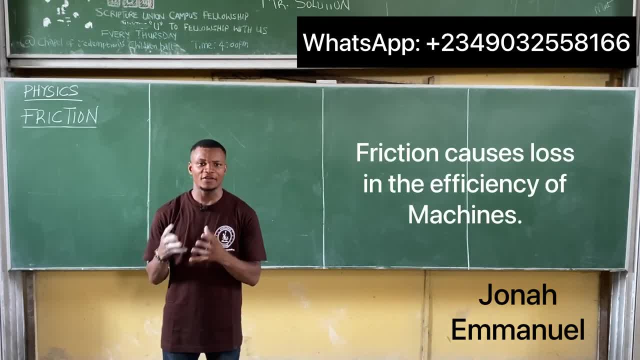 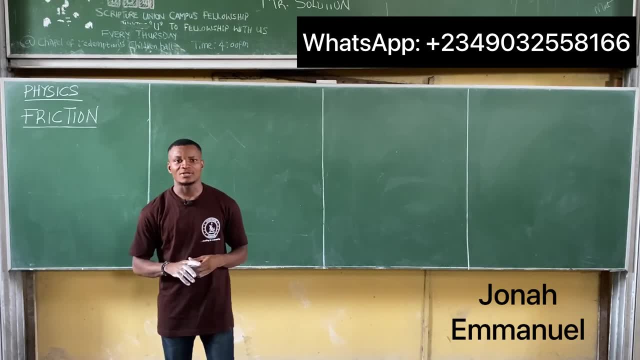 Friction causes loss in the efficiency of machines. We treated efficiency of machines in a previous class. There we said that the efficiency of a machine cannot be 100%. Why is this? Because some work is done to overcome friction. So, since some work or some useful work is being done to overcome friction, 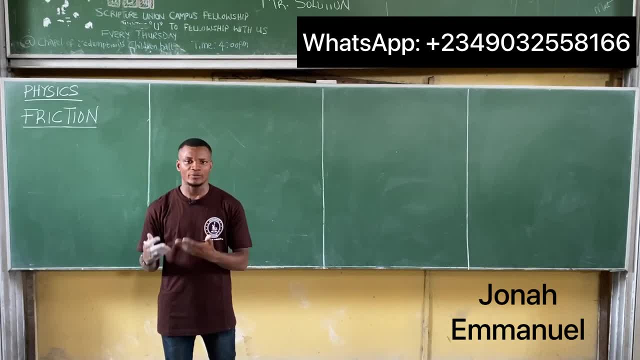 the efficiency of the machine cannot be 100%. That becomes its advantage of friction. It reduces the efficiency of machines because some work has to be done to overcome that friction. The third disadvantage of friction is that it causes the heating of engine parts And this is why if you ride a car for some time, by the time you park and you touch the 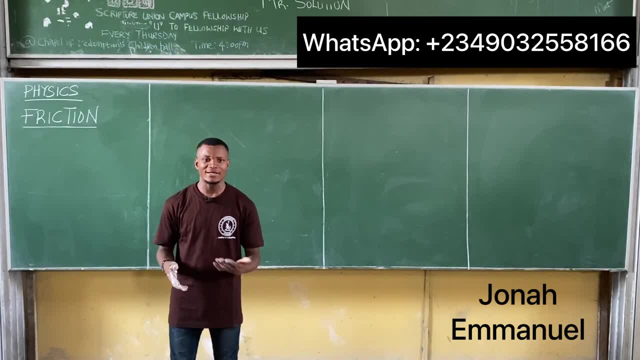 car, the engine part especially. it's very hot. Why is it hot? Because of what useful work has been done In terms of, or useful work has been done to overcome friction. Number three is that friction causes the heating of engine parts. 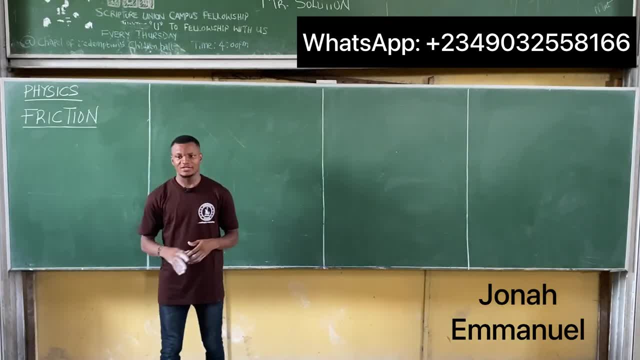 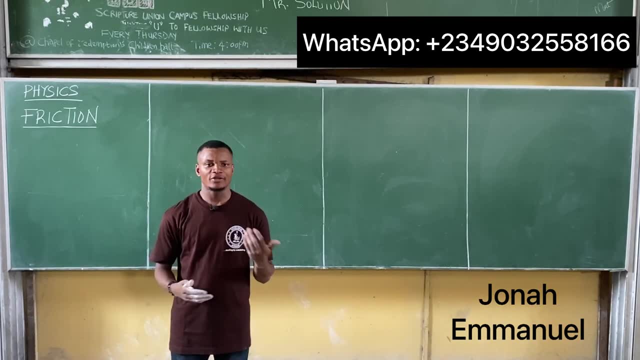 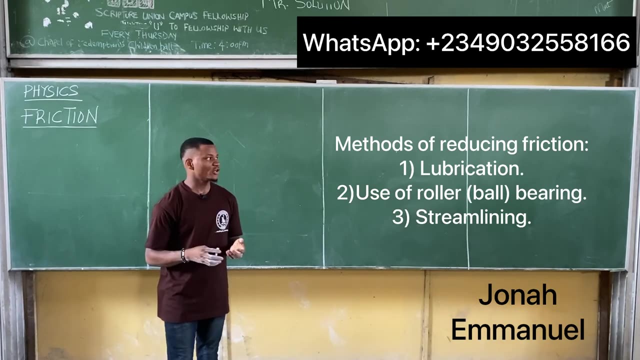 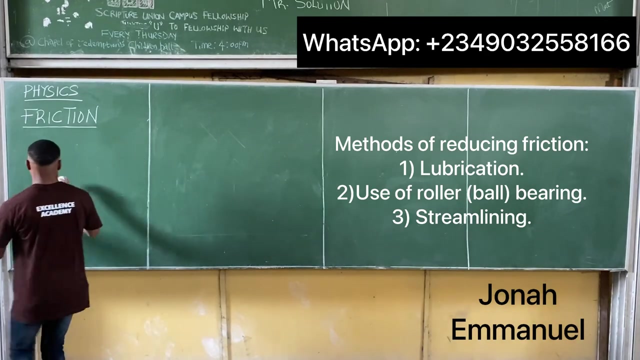 So these are like some advantages and disadvantages of friction. Finally, how can we overcome friction? We can overcome friction by number one: duplication. Number one is duplication. What is duplication? Duplication is simply a process of adding what we call lubricants. 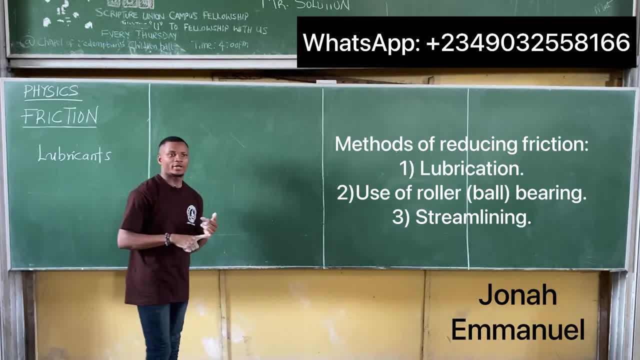 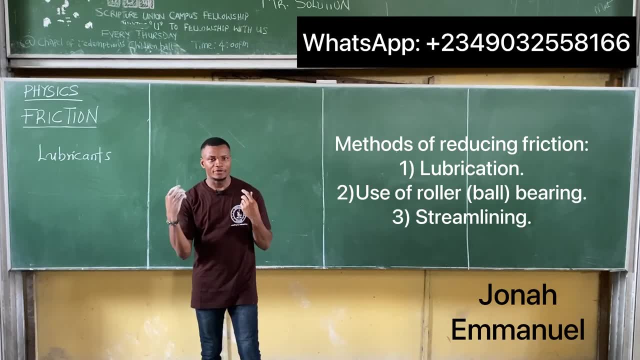 Lubricants. Lubricants such as engine oil, such as palm oil and some other things there to reduce the friction in machines, And this is why you add engine oil to your generator set, to your motor set and to your ATC.